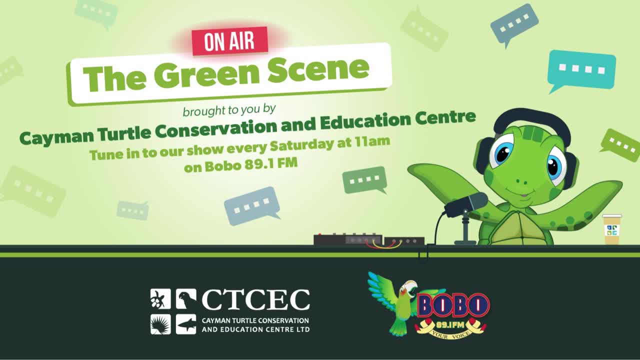 Enjoy a poolside barbecue, buckets of beer and daiquiri specials and a live DJ. It's Grill and Chill Saturdays at Cayman Turtle Center. Come and celebrate Cayman's culture and our national heroes at Cultural Day at the Cayman Turtle Center. 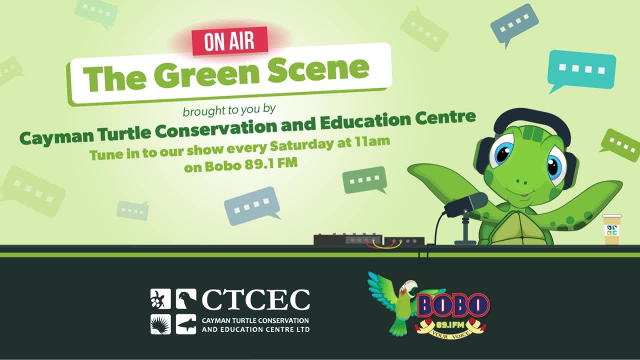 Monday, the 22nd of January, Cayman Turtle Center will be celebrating from 10 am to 4 pm with incredible deals for you and your family. Come and enjoy food and drink specials all day long, Swim with the turtles and fish in the lagoon. 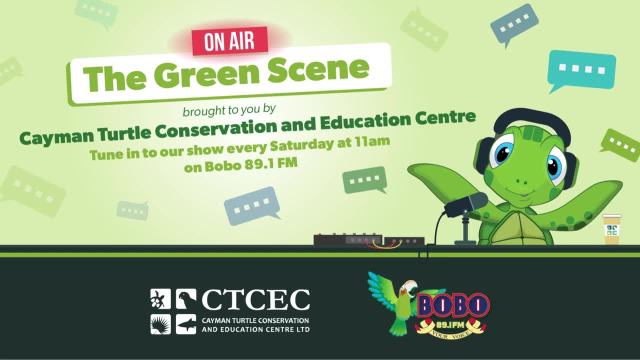 Enjoy the live DJ poolside and have fun with cultural activities throughout the park. Come and celebrate our heroes and immerse yourself in Cayman's culture at Cultural Day at the Cayman Turtle Center, Monday, January 22nd. Welcome to the green scene. 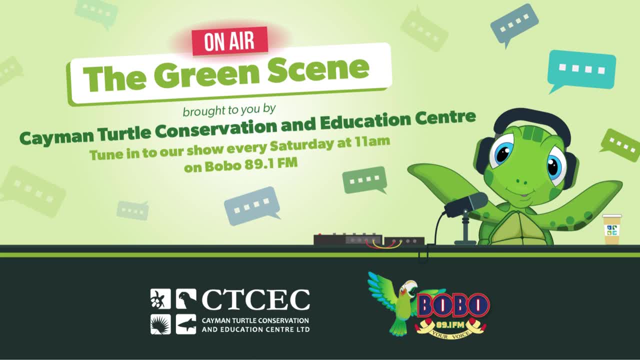 My name is Geddes Hislop. I'm the curator for terrestrial and education programs at the Cayman Turtle Conservation and Education Center. This morning I'm joined by my colleagues Dr Navi Babalal, who's our park vet. 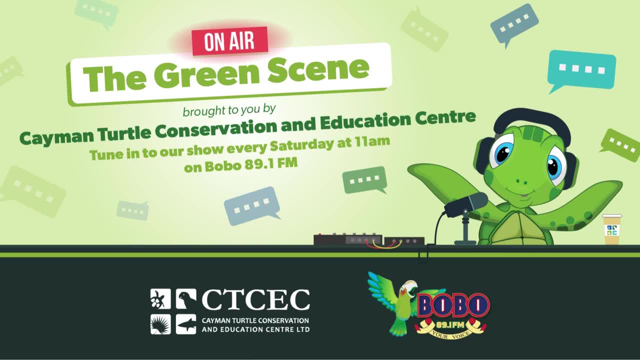 Mr Adam Jackson, the lead acarist, and Dr Gideon And our education officers at the Cayman Turtle Center, Shona McGill and Wendy Dandy. Today we're going to be talking about what do we actually do at the Turtle Center behind the scenes. 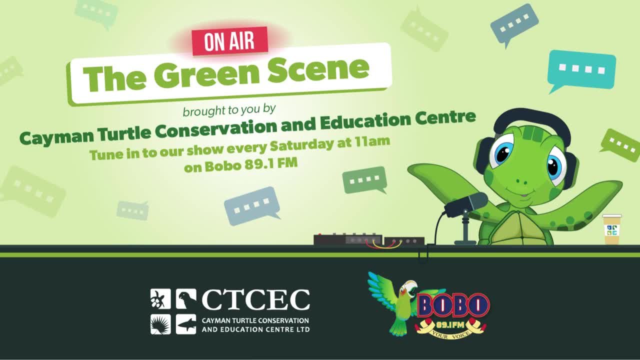 When people come into the park, they see turtles, they see swimming pools, but it's in our name. It's the Turtle Conservation Education Center. There's a lot of conservation work that goes on behind the scenes and we just want to make sure people understand that that's our purpose. 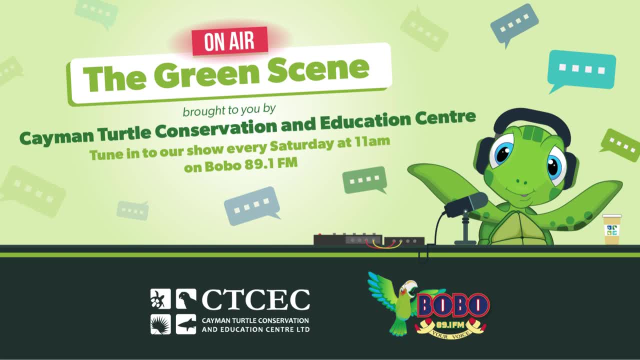 So we're going to get right into it. I'm going to ask Shona and Wendy to join me here. And guys, when we do our education programs, we do have a dedicated education programs team. We usually, with our presentation, we give people a bit of background on the company itself. 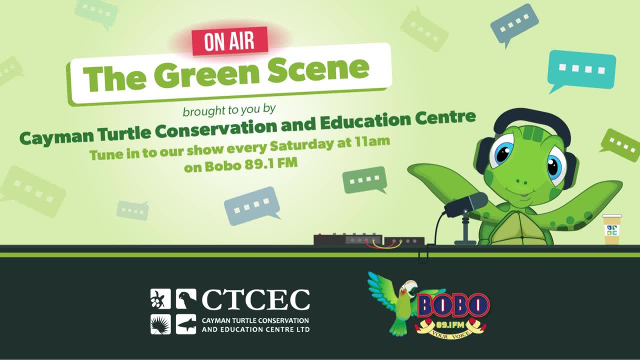 Maybe Shona can come in there and tell us what's the kind of things that we mention when we do these presentations. Yeah, so many people might not know that we've been around for a long time. We've been around for a really, really long time. 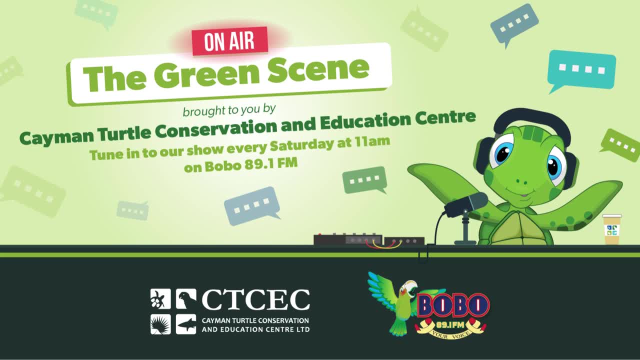 We've been around for about 55 years now. Our company actually started in 1968 as a company called Mariculture Limited and that was purely for the commercialization and breeding of the green sea turtles. So sea turtles here in the Cayman Islands were considered functionally extinct. 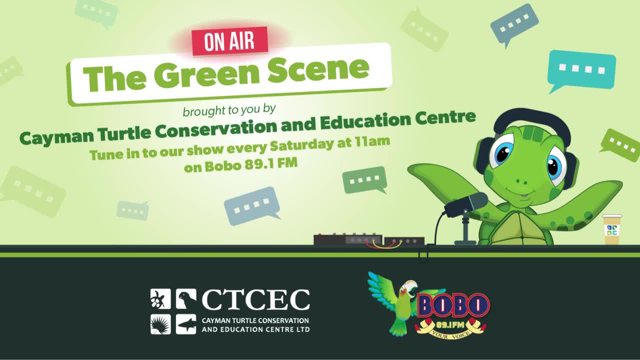 And that's just a really funny way of saying there weren't enough in the wild to continue the population. So Mariculture Limited started To breed these sea turtles And once we reached about 1980, we started the release programs as well. 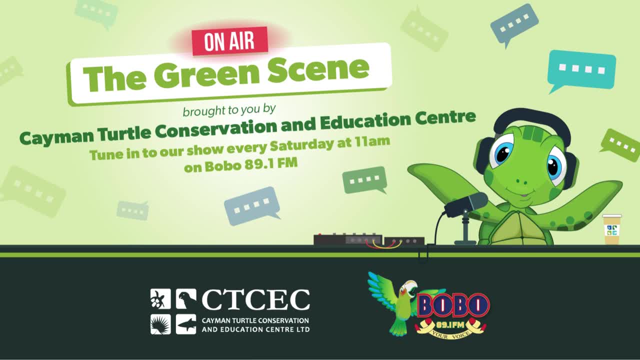 So we started putting the turtles back into the wild, But we went through quite a lot of changes. As you might know, right now we are not called Mariculture Limited, So we started off as that, And then we transitioned to Cayman Turtle Farm, once we were purchased by the government. 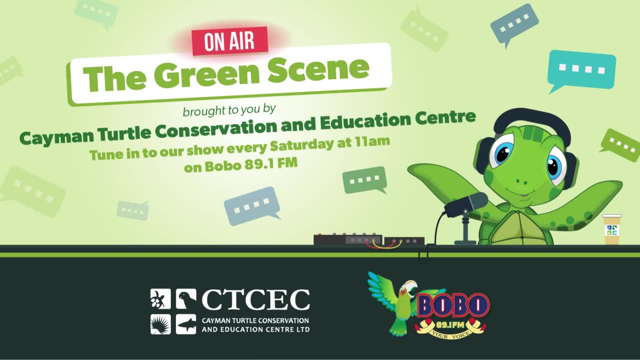 And since then we've gone through more changes, So we were known as Boswin's Bay, Which some people might know. We went back to Cayman Turtle Farm Island Wildlife Encounter. We then went to Cayman Turtle Center Island Wildlife Encounter. 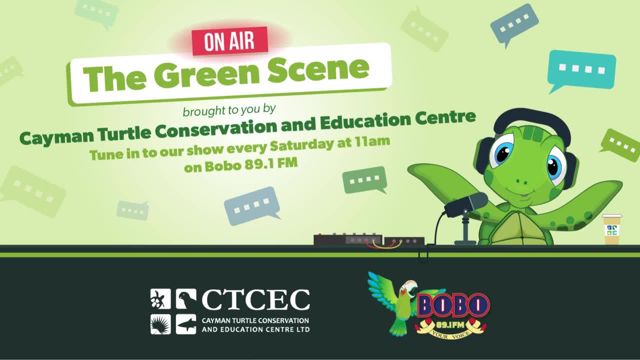 And now, with our multiple facets that we have of this company, we're fully known as Cayman Turtle Conservation and Education Center. Wow, that's a lot. It's a lot, That's a lot. But that means growth. It means the company has been evolving over the years, right? 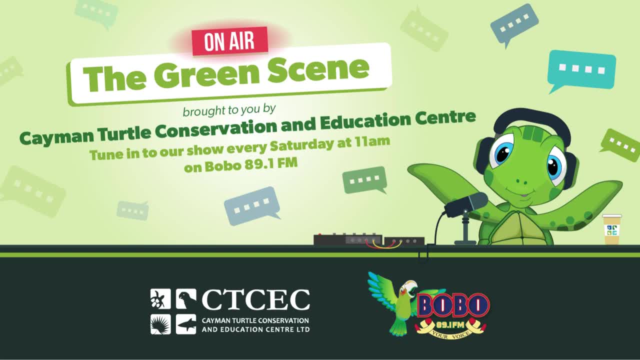 But today there's some accolades that we have That maybe most people might know about. Maybe you can give us a little background on that. Yeah, so there's quite a few. When people think of the Cayman Turtle Center, they generally think of a tourist attraction or a leisure attraction. 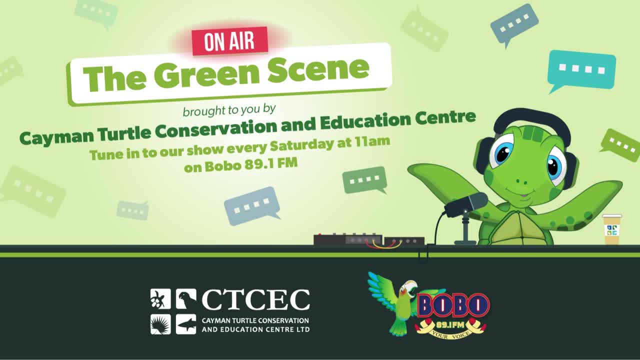 Some place to come and swim and just generally look at turtles. And the Cayman Turtle Center has accumulated quite a few accolades over the years, The first being that it is the largest land-based tourist attraction and the largest tourist attraction in general. 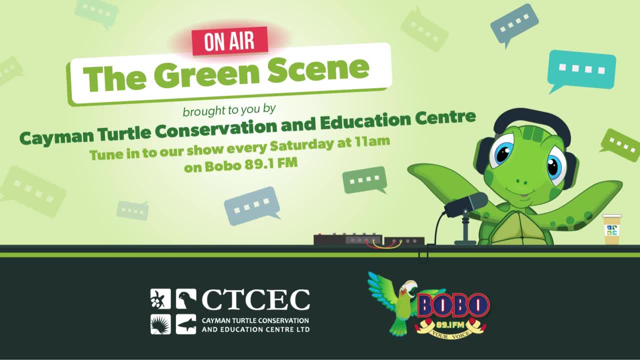 For quite a few years, we were back and forth with Stingray City, I believe in 2017, we prevailed over them as the number one overall attraction. So we have at least a quarter million visitors each year prior to COVID. So that's quite impressive as well for our tiny little island, as we know. 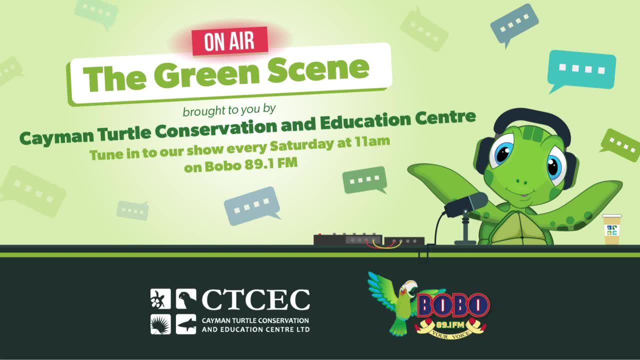 And also for Conservation-wise. our accolades are through the roof. We are the longest-running conservation program in the Cayman Islands And to date we have released over 36,000 turtles back into the wild. Wow, Right, So there's a lot of behind-the-scenes things that happens at the Turtle Center for years. 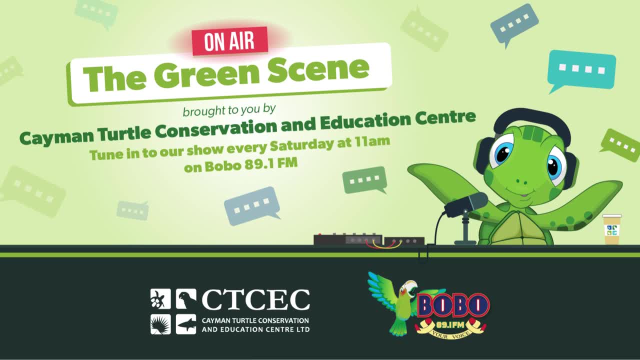 decades now that the public aren't quite aware of. And as the company has evolved, our conservation and education, our conservation efforts have evolved quite a bit as well, especially in the past five years. Yeah, that puts us just around the COVID time. 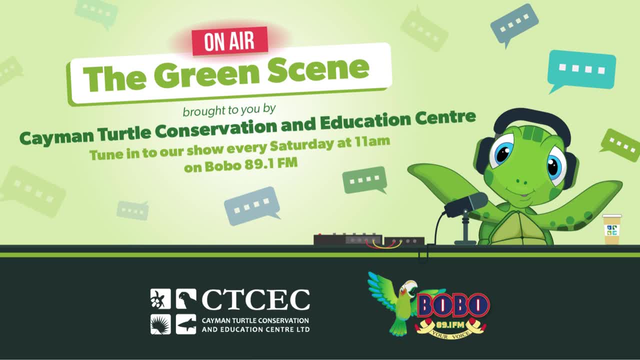 But yeah, so we have some things going on, a lot of things going on that people are not aware of, And I guess that's why we have this show, so people can know that the Turtle Center is more than just swimming in a pool and playing with turtles, which is okay, right. 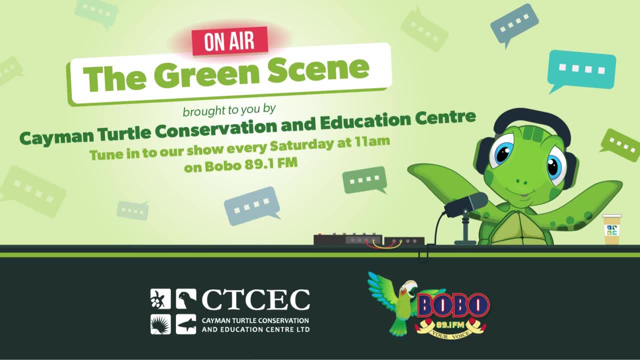 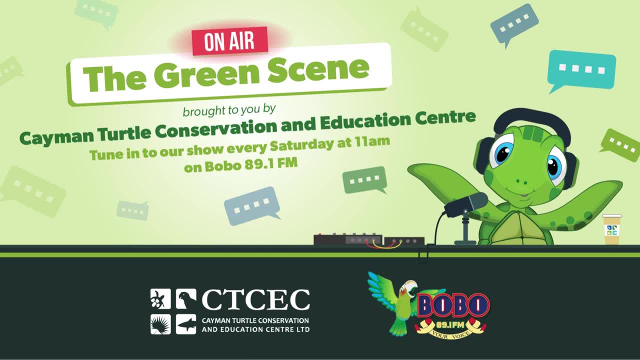 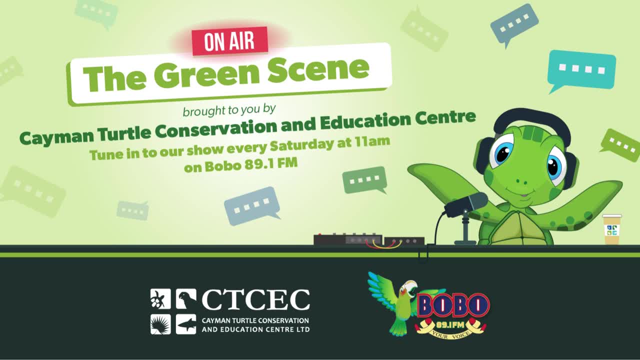 full-grown adults. But again, lots of conservation going on And I believe just prior to COVID we had completed a big study that gave us even more accolades. So you know, Shawny, you can give us a little background on that. 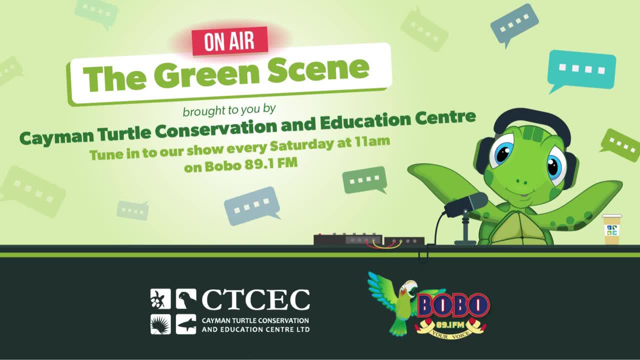 Yeah. So since starting our release programs in the 1980s, it was a little bit out of the up in air whether the turtles came back or not. The downside is we're working with the green sea turtle, which is a very, very slow maturing species. It can take them anywhere between 20 to 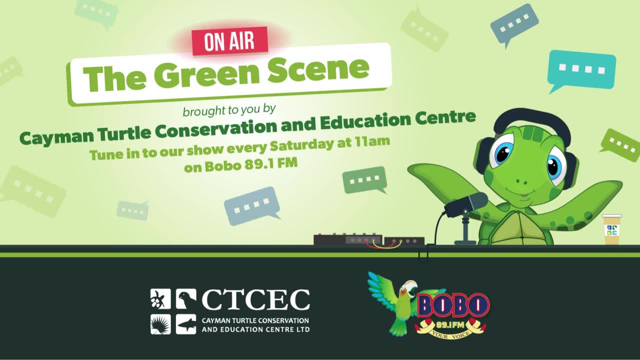 30 years in the wild to become mature. Now, the benefit of it is that females do a process called natal homing, which I always joke us scientists come up with really funny words to mean simple things. So all natal homing means is that that female will come back to the beach she was born on. 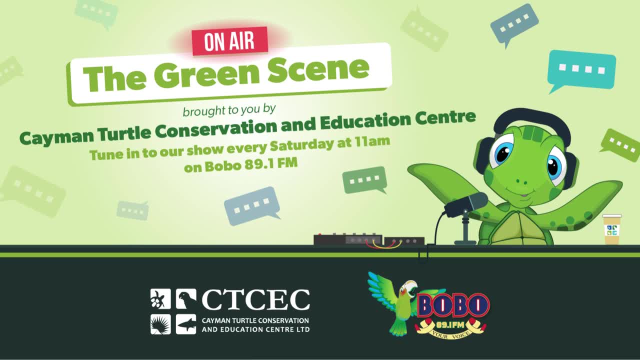 or released on to lay her eggs. Now, because of this, we had to wait a little while to get those results, but we did a huge collaborative study with universities like University of Barcelona and University of Exeter. We partnered with Department of Environment and a few other. 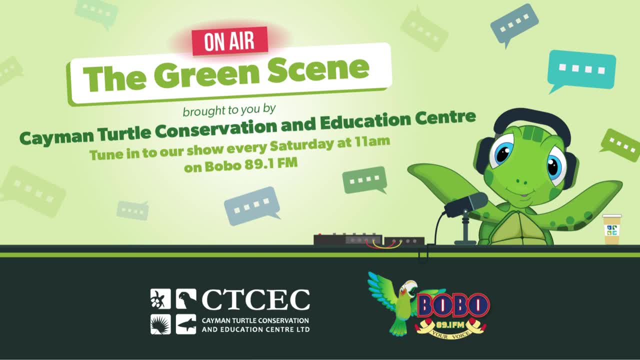 places as well, And it was a huge study over a few years that we did a huge collaborative study with universities like the University of Barcelona and University of Exeter, And we partnered with Department of Environment and a few other where we took the DNA of the wild nesting green turtles here in the Cayman Islands and also took 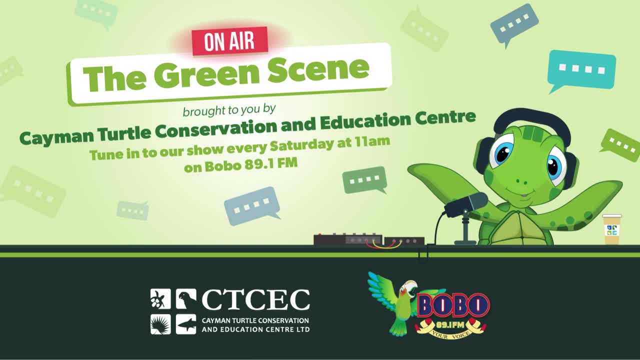 the DNA profiles of our turtles at Cayman Turtle Center, And what we found out was that 90 percent of the wild nesting turtles in Grand Cayman has DNA related to the turtles at Cayman Turtle Center. And what's even more shocking, I should say, is that later on there was an update that showed: 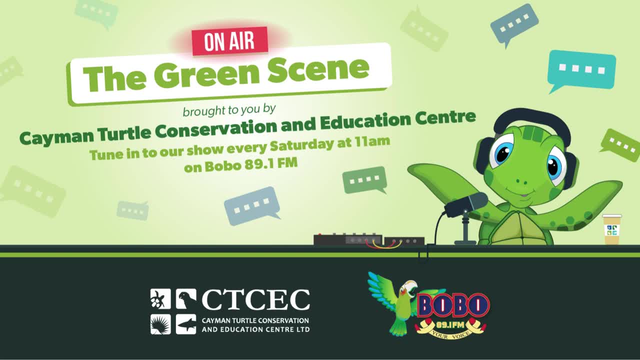 almost 80 percent of the nesting turtles in Little Cayman had DNA related to our turtles as well. Wow, in Little Cayman. In Little Cayman, So that means you're releasing turtles in all three islands? Yeah, so not many people know about that. We've released turtles in both Cayman, Brac and Little. 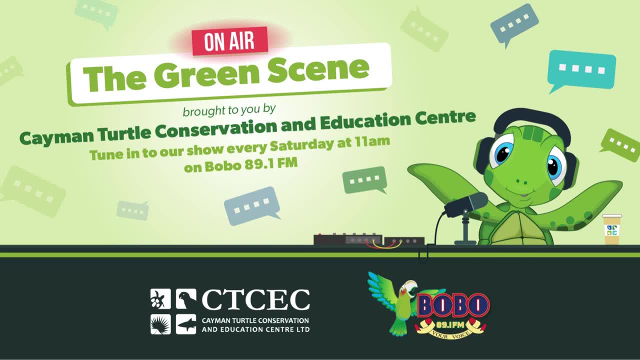 Cayman as well, in partnership with Cayman Airways. Oh, shout out to Cayman Airways. Yeah, the turtles didn't swim there themselves. Cayman Airways very generously helped us get the turtles over there and we've been releasing them. But it's not just the Cayman Islands. Our turtles have been tracked as far north as the Florida Keys. 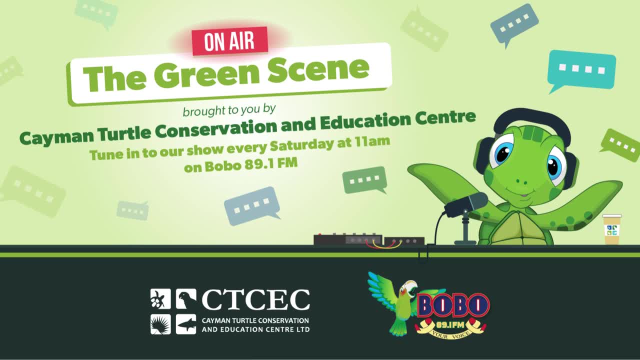 and as far south as Venezuela. They don't have to stay here. So that means we're also affecting the wider Caribbean as a whole. Oh yeah, so yeah. so those releases don't just mean the turtles here, that are the only ones that are being affected. but yes, why the Caribbean? Venezuela? 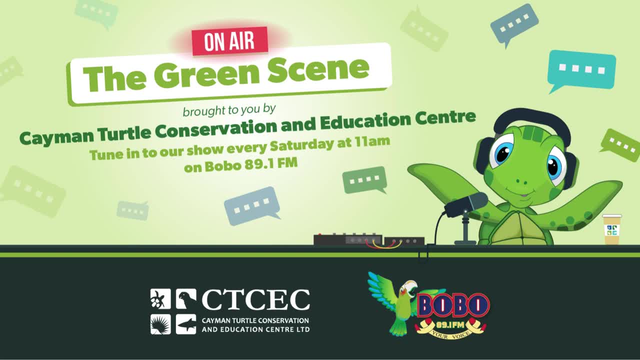 that's a long way from here. That's a very, very long way. Yeah, that's a. really That's a long way from here. That's a very interesting And because of what work we're doing, we can say things like that, because we're actually tracking these animals. 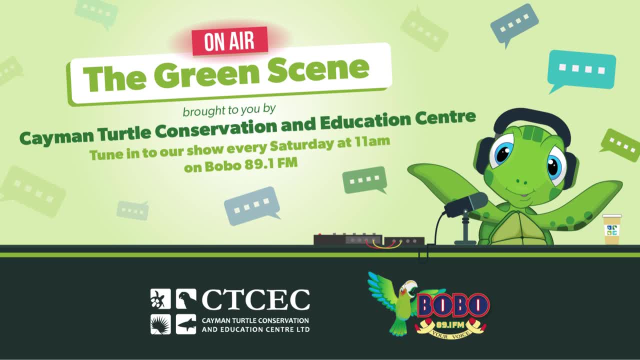 This is great. Well, we've come through all these accolades and it's definitely a team effort, because that didn't happen on its own. There are so many departments at the Turtle Center that work together to make the company work just like any other big company, And I think most people. 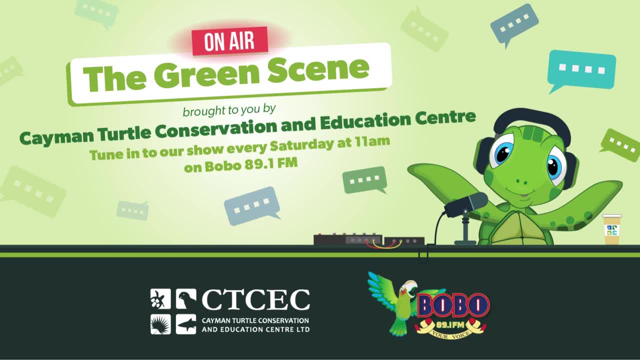 They see some. they don't see everybody, but we have- for example, just so that you know, we have- a section called the Animal Programs Department, and we're the ones- I guess we're part of it. they're the ones- that actually deal with the animals themselves. 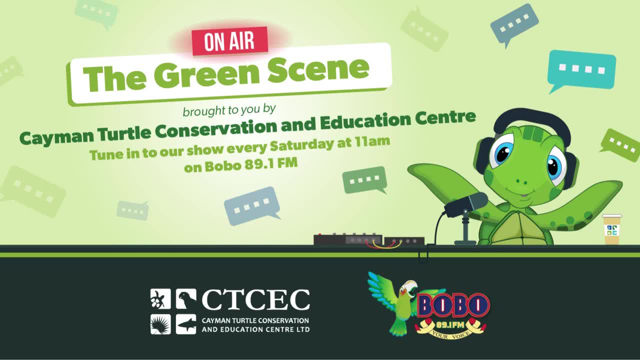 Like a couple of our guests today from the Marine Department, as we say, that's anybody, anything that swims and has fins. And then we have the Turtle Husbandry, which is, of course, Turtle Center. We must have people. we have a whole department dedicated just to turtles themselves. 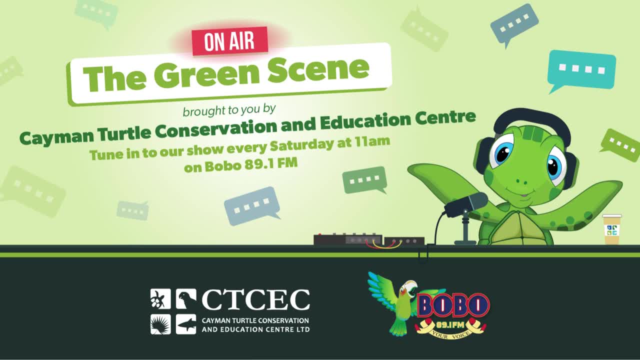 The Terrestrial Department. that's my section, Anybody anything with legs and feet, because we do a lot more than just turtles. there at the Turtle Center- And most of you might not know- we have a dedicated Education Programs Department And you know it's more than- and again, that's more than- just dealing with schools. 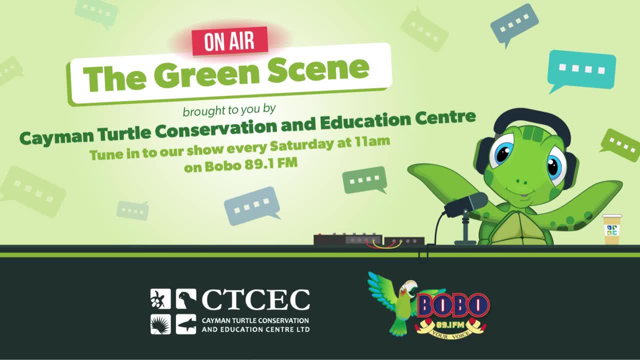 although we do get a lot of schools. But we'll get into that a little later. Other departments include Tours, our Lifeguards Department. We have a Food and Beverage because we have our Schooner's Restaurant and our Silver Thatch Cafe. 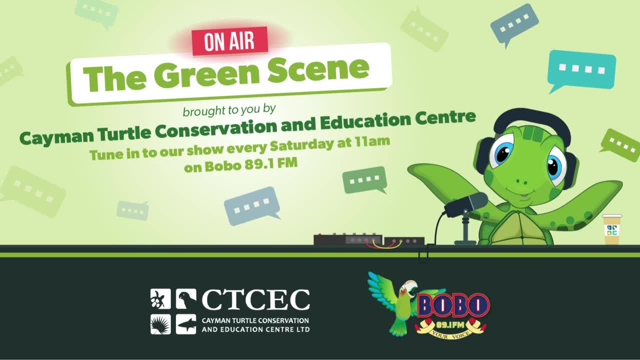 Retail Department, the Splash Gift Shop, which I understand is very popular, And our Customer Service Department And, of course, the Admin. Somebody has to make sure all the finances and things like that keep running, But everybody, Everybody there, contributes to conservation directly or indirectly. 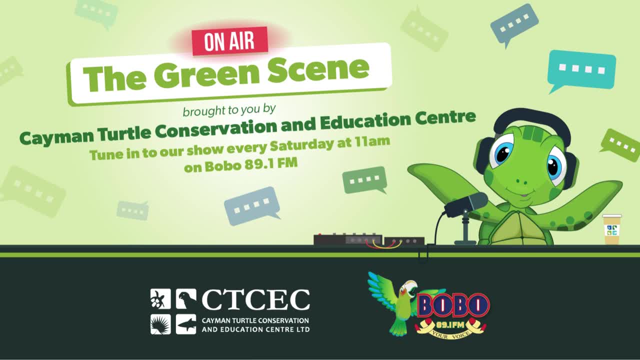 That's the thing. We want people to understand, that. So I guess we can discuss a little bit more about that, And maybe we can start with the Education Programs Departments, Because they're dealing with animals. It's kind of obvious that, yes, all these releases and everything. 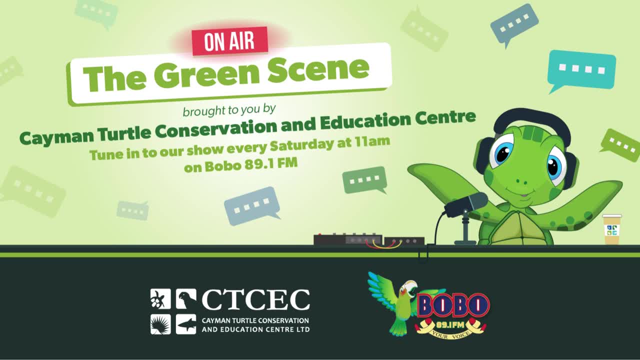 there's a weird team that makes that happen. So what we're going to do is we'll take a short break And when we come back we will get into discussing the various departments that actually work with animals, So our Turtle Husbandry, our Marine Departments, our Education Programs and our Terrestrial 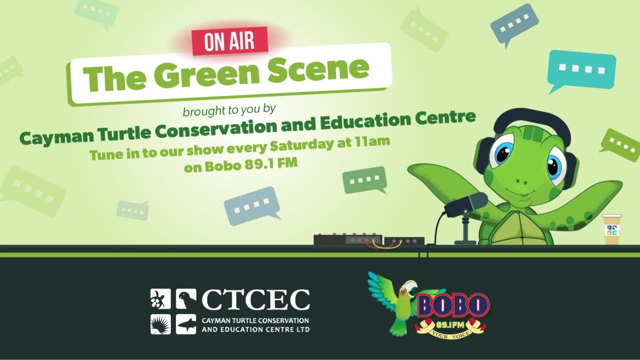 So you're listening to Green Scene on Bobo 89.1 FM And we'll be right back. Hi. you're listening to the Green Scene on Bobo 89.1 FM, brought to you by the Cayman Turtle Conservation and Education Center. 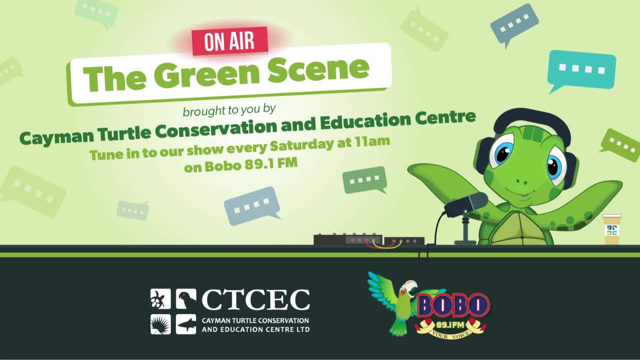 I'm Jennifer Robinson and I'm the aquarist. We'll be back in a few moments. Come and celebrate Cayman's culture and our national heroes at Cultural Day at the Cayman Turtle Center, Monday, the 22nd of January. 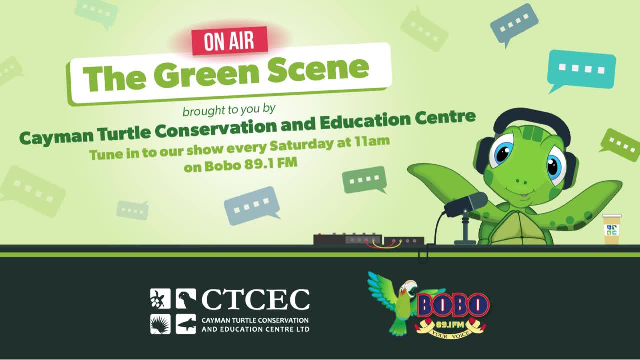 Cayman Turtle Center will be celebrating from 10 am to 4 pm with incredible deals for you and your family. Come and enjoy food and drink specials all day long. Swim with the turtles and fish in the lagoon, Enjoy the live DJ poolside and have fun with cultural activities throughout the park. 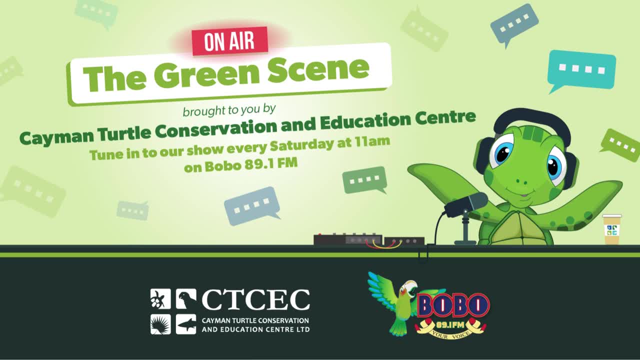 Come and celebrate our heroes and immerse yourself in Cayman's culture At Cultural Day at the Cayman Turtle Center, Monday, January 22nd. Looking for something fun and different to do with the family, Join us at the Cayman Turtle Center for Grill & Chill Saturdays. 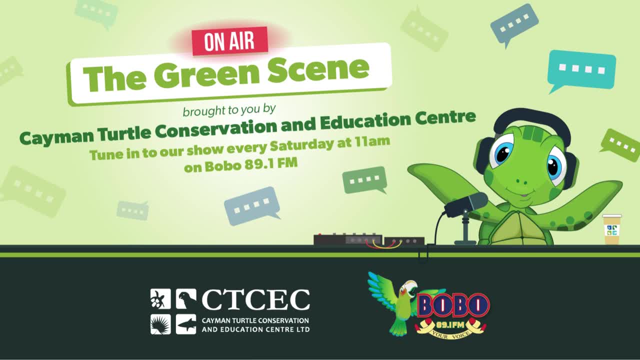 Every Saturday from 11 am to 3 pm, Enjoy a poolside barbecue, buckets of beer and daiquiri specials and a live DJ. It's Grill & Chill Saturdays at Cayman Turtle Center. Welcome back to the Green Scene. 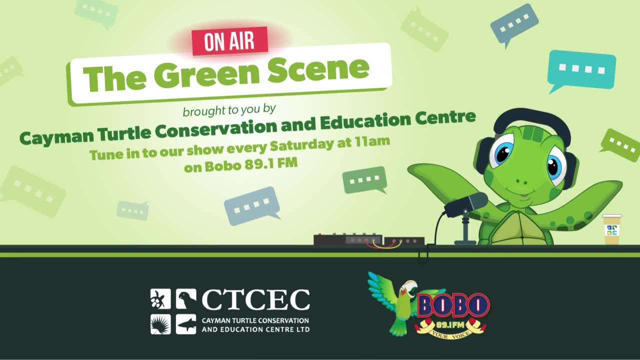 My name is Gedis Hyslop. We are here discussing what we do at the Cayman Turtle Center. behind the scenes We've been sitting discussing here with our colleagues, education programs officers Shauna McGill and Wendy Dandy. We just established that the Turtle Center has a lot of accolades going on. 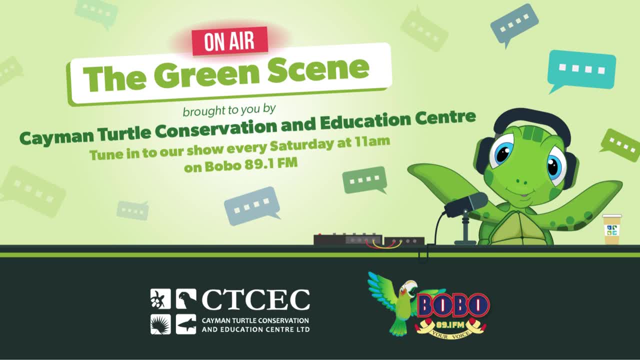 And besides just being a place to see turtles and swim, there's a lot of conservation work going on behind the scenes, And we're just going to start discussing some of the departments that helped make that happen, because it is a team effort, And one thing people might not know is that we have 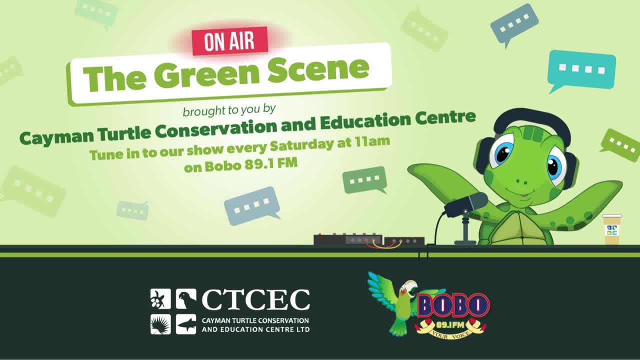 we have a dedicated education programs department and we have education programs officers. That's what we're talking to right here. So Wendy and Shauna are two education programs officers here at the Cayman Turtle Conservation Education Center. Why don't you guys introduce yourselves, give people a little background and you know. 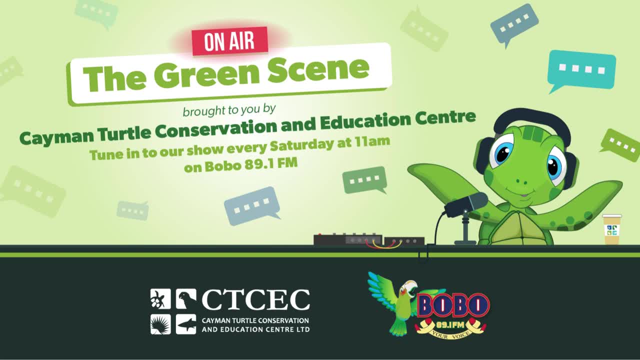 your qualifications and what it's like being an education programs officer. So, Shauna, why don't you go start? So I always knew I wanted to work with animals and I sort of facilitated that through volunteer programs, volunteering with places like the Humane Society. 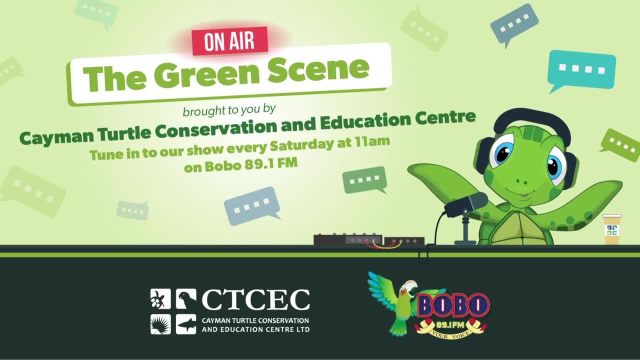 doing internships at the vet, very quickly realizing I didn't want to be a vet but solidifying the fact I wanted to work with animals. So I made the decision to go to university in the UK. I went to Anglia Ruskin University in Cambridge and I studied animal behavior and welfare. 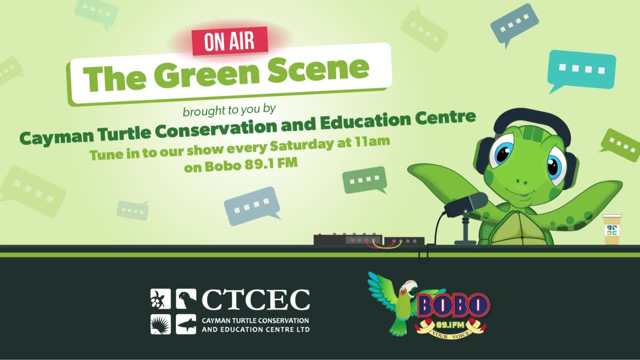 So a deep dive I went to the mental capacity of animals and why they do the things they do, which is actually very beneficial. It's very in depth, but it helps me at least understand animals just a little bit on a daily and see why animals are behaving the way they do. 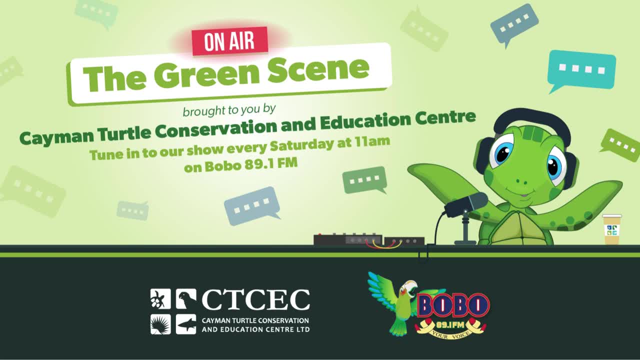 I hope you understand some people too. Yeah, definitely Okay, And Wendy Okay. Um, well, I started school in the Cayman Islands. Um, I went to school in the Cayman Islands. Um, I went to school in the Cayman Islands. 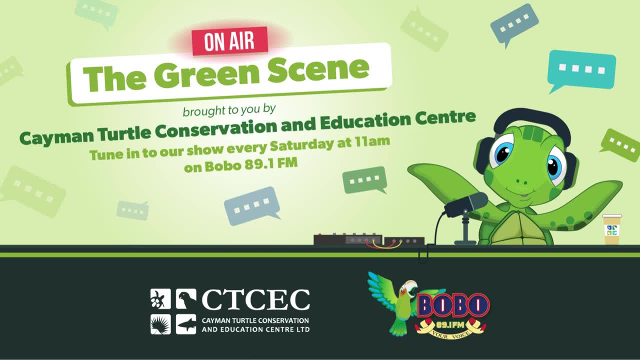 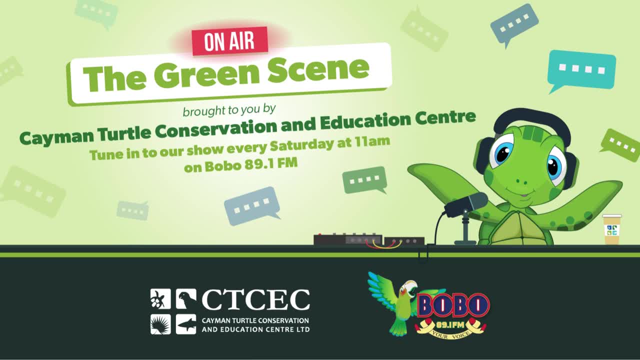 um green development side of things, so a more well-rounded view in. so I started off with animal sciences and ended with environmental policy in green buildings. So both backgrounds are, you know, yeah, science and science and animals to a point and but education programs. most zoos and aquariums around the world have education departments. So both backgrounds are, you know, yeah, science and science, and animals to a point, and but education programs. most zoos and aquariums around the world have education departments. So both backgrounds are, you know, yeah, science and science, and animals to a point, and but education programs. most zoos and aquariums around the world have education departments. So both backgrounds are, you know, yeah, science and science, and animals to a point, and but education programs. most zoos and aquariums around the world have education departments. So both backgrounds are, you know, yeah, science and science, and animals to a point, and but education programs. most zoos and aquariums around the world have education departments. So both backgrounds are, you know, yeah, science and science, and animals to a point, and but education programs: most zoos and aquariums around the world have education departments. So both backgrounds are, you know, yeah, science and science and animals around the world have education departments. 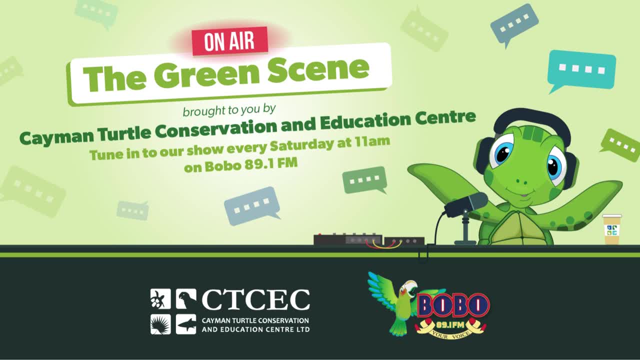 transition from. I mean, that's a transition. just just having a degree doesn't make you an educator. what else did you have to do? So I initially started working at Cayman Turtle Center as an aquarist. so I was with the marine department and that sort of facilitated my learning working. 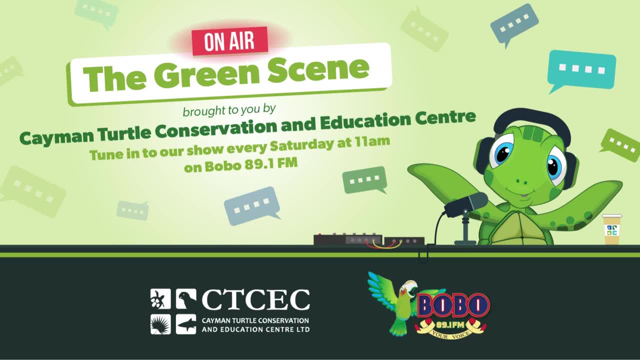 directly with animals, but it's not just going out and getting a degree. you genuinely need to facilitate learning all throughout animals. Animals are constantly changing. we're constantly learning new things about taking care of them, how they behave. there's a reason why we're science and scientists: because it's always changing. people are always investigating, so, even though 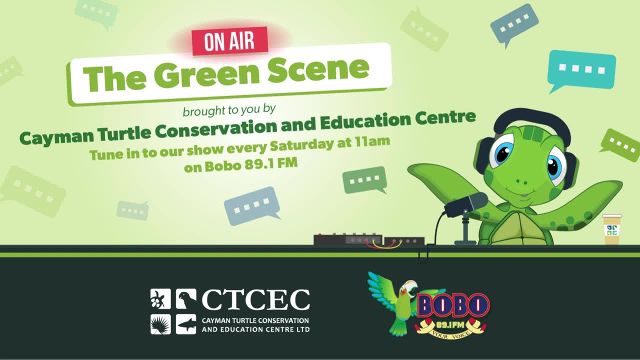 we're working in the departments. we're constantly facilitating our own education as well, so we have multiple programs that go on. we have the aquarium vet course, which teaches us more about fish and marine animals and their physiology and how they behave and how to take care of them. then we also have the San Diego Zoo Global Academy, which focuses more on the care of 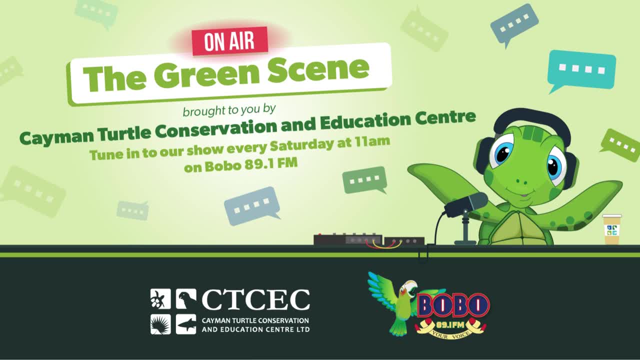 zoo animals, but also goes into depth about educational programs, natural disasters and how to recover over that. so it is quite a deep depth course. Yeah, yeah, so that that's how to. so, yeah, I think that that helped you focus. what you already know is doing those courses. 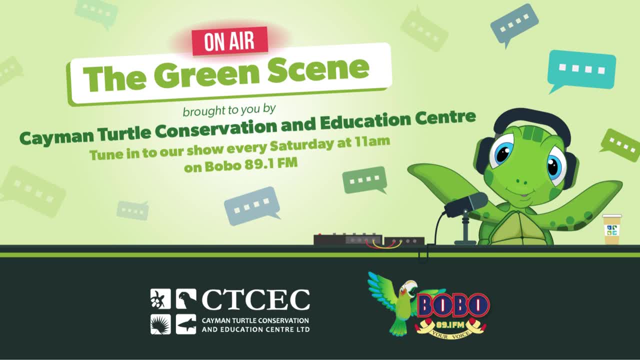 Basically, yeah, just fine tune on how we bring across and present information in a way that helps people retain. Yeah, well, that's why I prefer to call it interpretation, because because we do have a lot of, we do have scientists, a lot of scientists working at the center, and 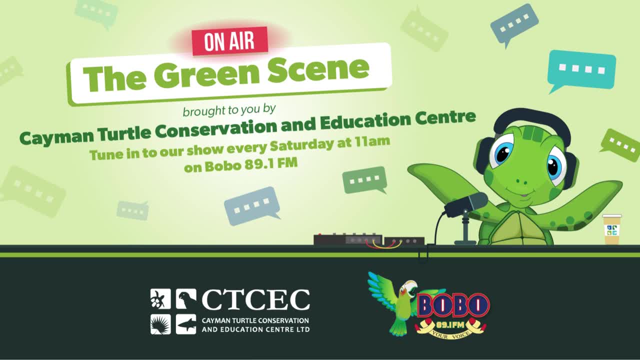 sometimes, I think Shauna might have mentioned earlier. you know, science has a funny ways of saying simple things right, makes it sounds really complex. so it's a simple thing. so it's kind of like interpreting another language and breaking it down to different levels. so so for the education. 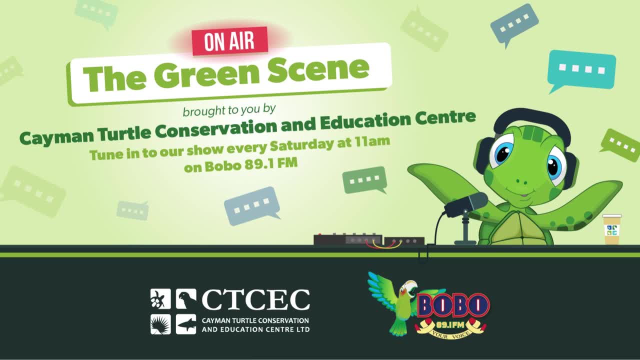 programs when think education movies, but most people think about schools. right, I know we do have a lot of schools visiting the center. tell us about that. yeah, so we definitely have a lot of schools visit our Center from various schools across the island, different age groups as well. so our educational 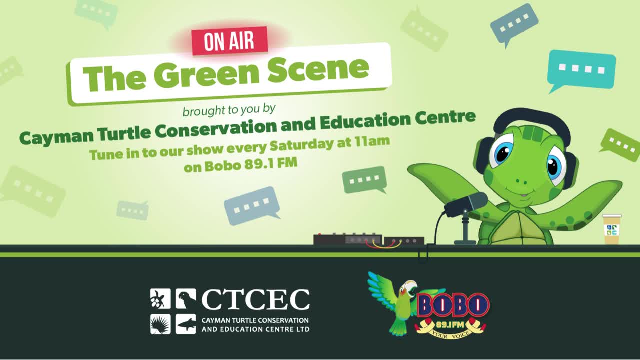 programs and educational talks don't just focus on school age children- I'm putting that in bunny ears. so we don't just do primary school and high school, we also do university level two. in fact, we don't just focus on schools here in the Cayman Islands. we also have many schools from other countries, like places. 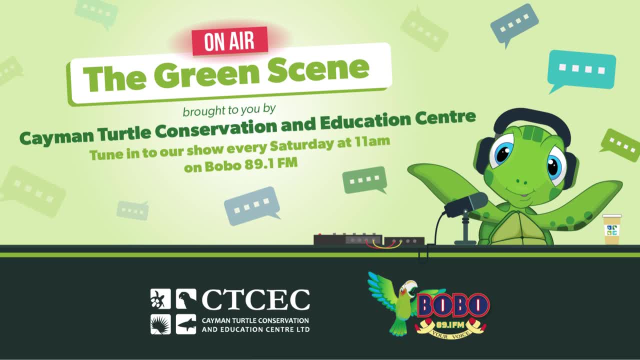 like Canada and the US that either come here on vacation and visit our center or we either do virtual tours with them as well. say what you want about covid, but the one benefit of it is that it made us work and find different ways to reach a different audience, because they couldn't. 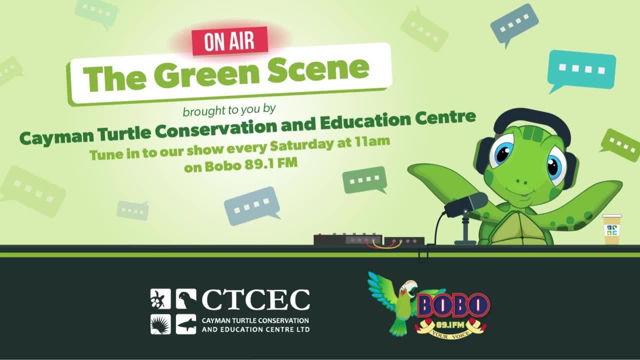 come in. so that helped us enhance our educational programs and we were able to do more virtual outreach to not only places here in Cayman but across the world too. oh, yes, let's say something for virtual technology and besides, and you said, yeah, we do just. we don't just do schools. uh, don't we do? 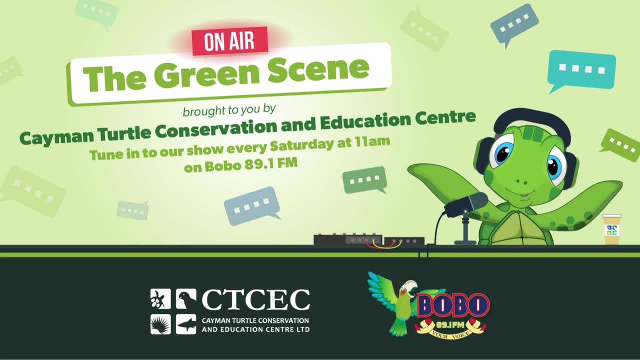 we do corporate outreach, right, Wendy? yeah, so we have a dedicated corporate outreach program as well, where we come and do lunch and learns. we have something called act talks, which stands for animal conservation talks, and right now we have two that we are that we present. the first one is called how many. 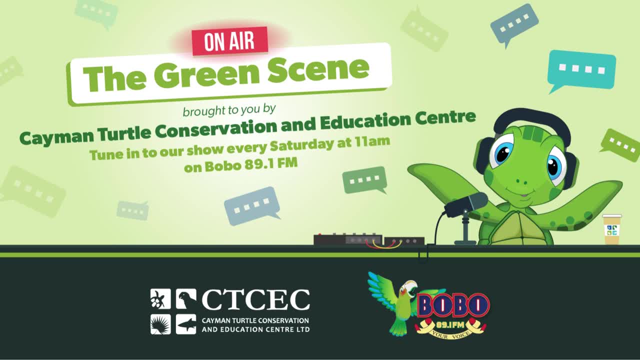 came home and the second one is entitled iron men and wooden ships. so basically it's um two educational talks that our team has put together to present to the public. we try to extend our educational reaches outside of the park. there's a lot of people who don't know what's happening. 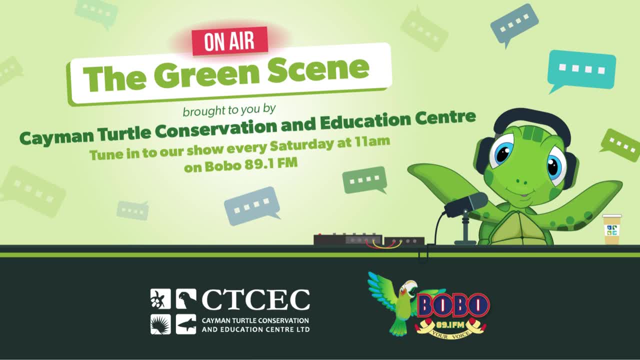 behind the scenes and a lot of people who don't know the history of our islands as well in terms of the green sea turtle. so we try to get out there- and we've done quite a few law firms, a lot of other admin companies as well- and we come in for about an hour, do a lunch and learn. we've had a really great feedback and 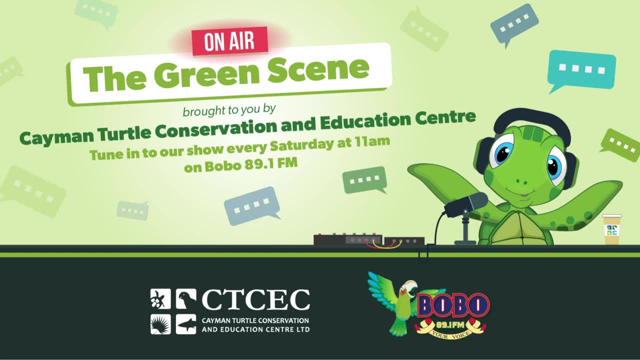 attendance so far, since we've been doing these talks. so for those of you who are interested, um, you can get in touch with us at info, turtleky, mm-hmm. and for the schools- schools visiting- how do they get in touch with us? yeah, so if someone is listening, 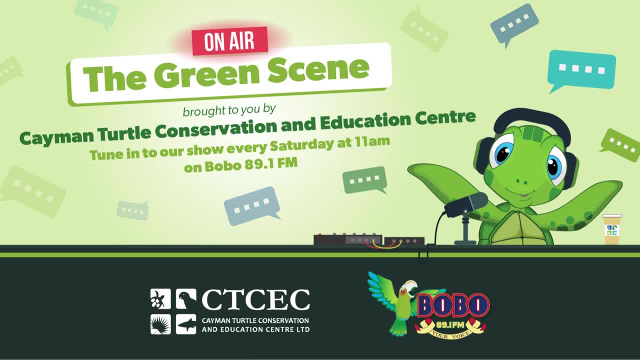 who wants to get their classroom in touch with us. all you have to do is email. school tours at turtleky. yeah, all right. so apart from the people who visit- well, we have our schools, you have our corporate- people will reach out to them. and yeah, because while we're educating, 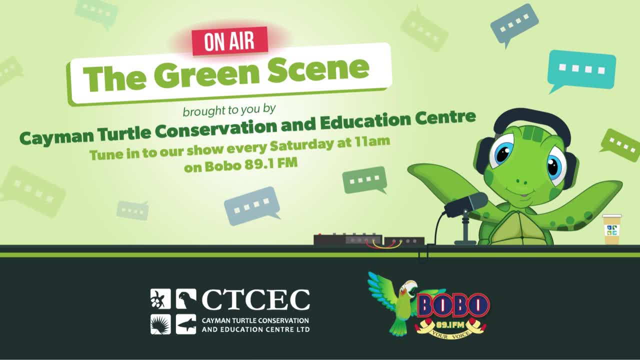 the younger, the next generation. we still have people that are here making decisions and I guess our education outreaches to make sure that they're making informed decisions. at least they have that, that background, that environmental focus in mind. uh, but the park itself is, it's like I said, it's in. 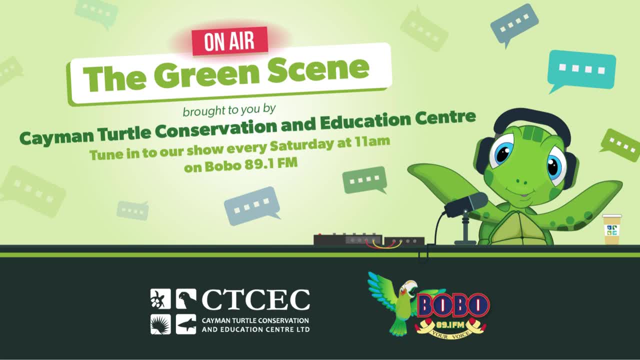 the name total conservation Education Center. what else does education programs do? yeah, for example, I think it's really important to note that it's not just schools coming in that are getting education from us. anyone that walks through our doors is technically getting education from us is technically getting education from us. anyone that walks through our doors is technically getting. 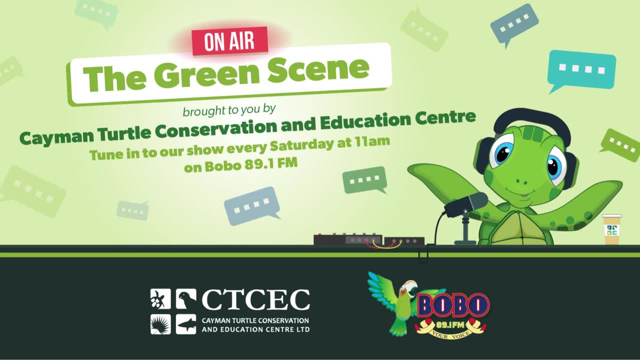 an education on our company, but also the green sea turtle, as well as all other animals we have at our park. yeah, yeah, so sorry. we do that by um doing daily talks, um shark talk, for example. um, we also have weekly talks, like crop talk as well. um, when it's breeder season, we have our hatchery talks. 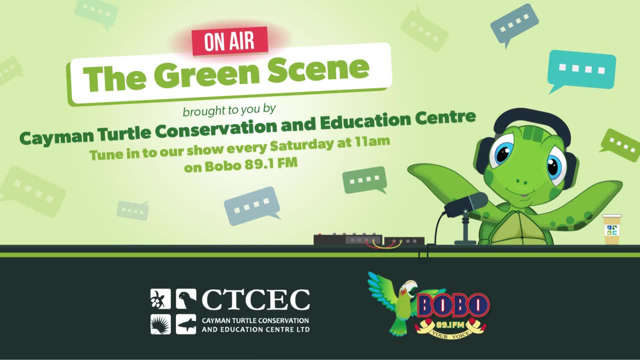 we've trained and gone through scripts with our tour guides, both internal and external. um. we have extensive signage that has been pre-written and approved by our educational officers. so there's quite a lot of thought and more detail that goes into our educational outreach than people realize. every day we're interacting and getting some kind of educational. 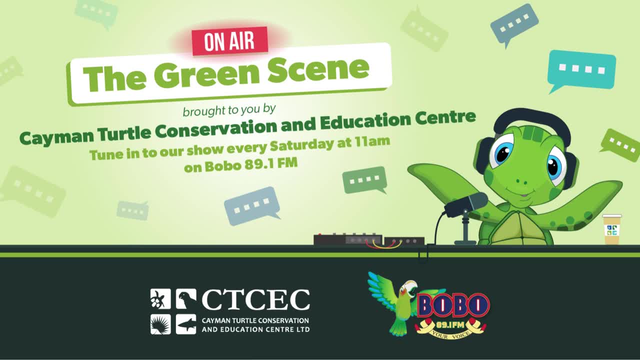 facts out there, yeah, and you should point out that also our purposes. everybody's an educator, obviously our tour guides. as soon as you create an open access website, or at least our tour guide, go hack, test out the different pieces of insane activities you just saw right now. 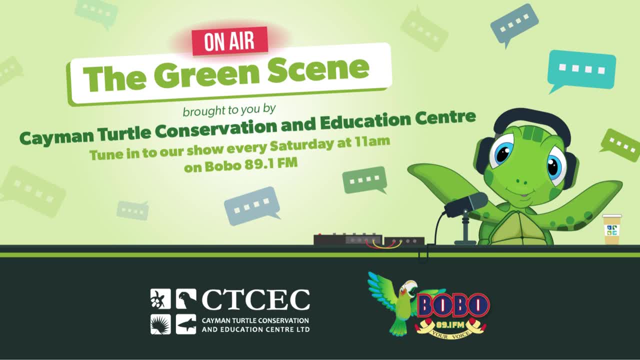 I saw the went Gala where the park, Limuru Еще the park, so it's actually the park that I meet with my friends and生活, kita for our beside tour guides and both our on-site tour guides as well as the ones that are up. there are independent operators that bring people to the park, but, uh, our own staff, our animal programs, people, the, the across the keepers, even the lifeguards, and so on. to an extent, everybody gets an, everybody gets information from us. so, yes, education is very important. it's its to make sure we're keeping everything up-to-date and in that, 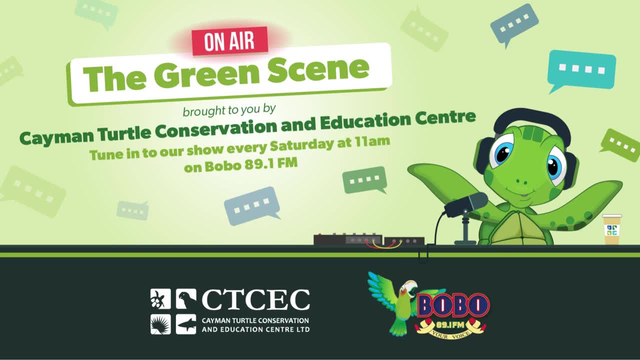 I think we also work with our marketing department as well. right, Oh, most definitely Yeah, Very closely with our marketing department? Yeah, because a lot of information going out on our websites and our social media platforms. they all have to be kept up to date. 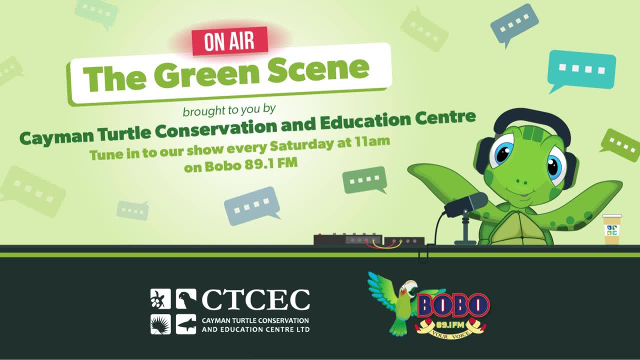 But one of the things where people see you guys out in the public, well, I'd say, besides school visits, is the Twitter releases. Tell us something about that, because you have different types of Twitter releases, right, Yeah, so, honestly, being an educator has so many branches. 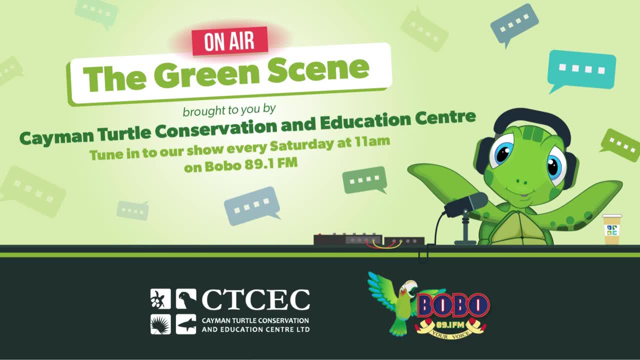 including Twitter releases, which in itself is a whole event. So us as educators, we also act as the Twitter release coordinators. So we're there helping plan how our Twitter releases are going to go out, but also, more importantly, giving the educational talks. 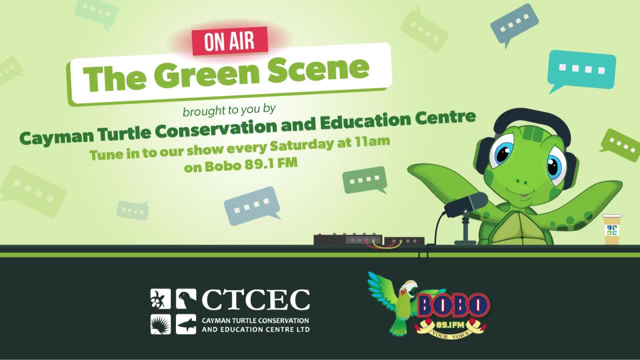 at each and every single one of these releases. So, whether it's our Nest Trans location, where we take our own uncapped-to-bred eggs and implant them on local beaches, whether it's our hatchling releases, when we take them out at night and release them from the beach, 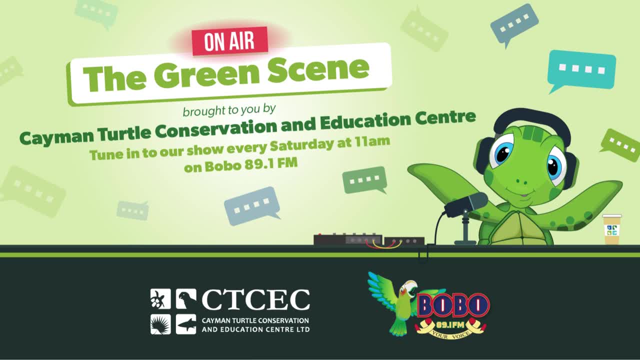 or when we take them out in a boat to sargassum rafts and release them, or, finally, whether it's our Head Start at Twitter releases. It's sort of our job there to ensure that all the information going out to the public about our programs is accurate. 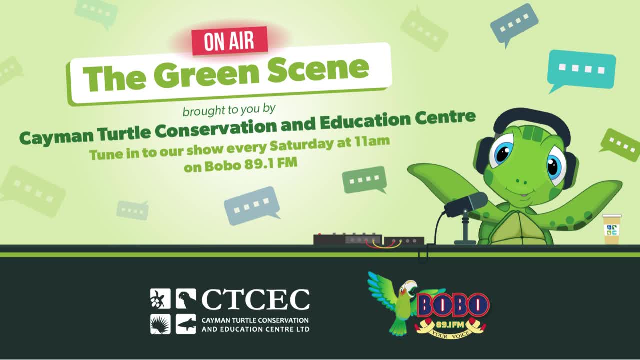 but also answering any questions they may have. Okay, That's a lot, It is, Yeah, it is, But, like I said, it's in the name. so it's a very important component of what we do at the Taman Tulu Conservation Education Center. 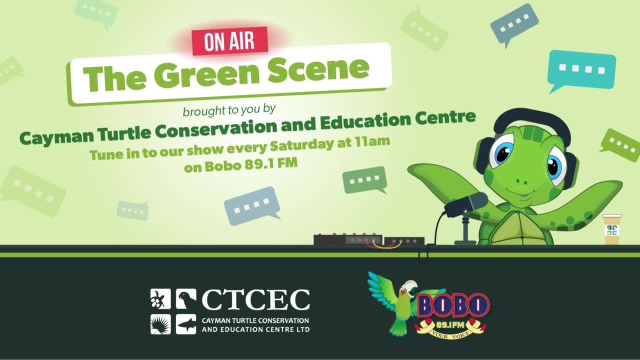 And most people. and, of course, education is probably one of the most important tools that we have for conservation, Because we want people to go away informed, making the right, so they can make decisions, their environmental decisions, their own decisions, keeping things in mind that do with our environments. 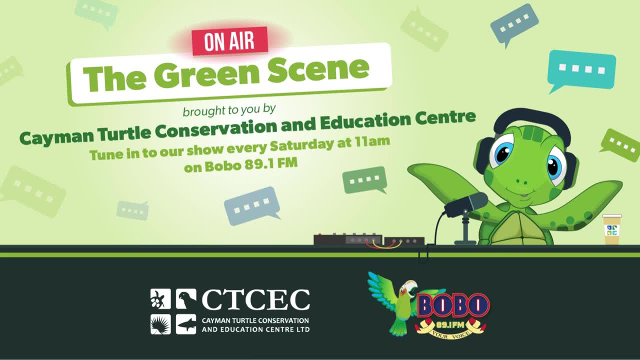 and our animals. Yeah, there's a quote and I'm going to paraphrase this because I'm not going to remember it off the top of my head, but it goes something like: you protect what you understand, you understand what you're taught. 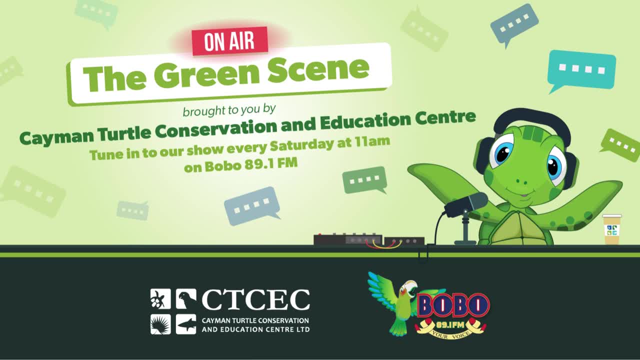 And so it's sort of our job to get the information out about the species to also help improve the conservation of the species we work with as well. Mm-hmm, definitely, And really important to have that information accurate. So being an education officer doesn't mean you're just spouting out things. 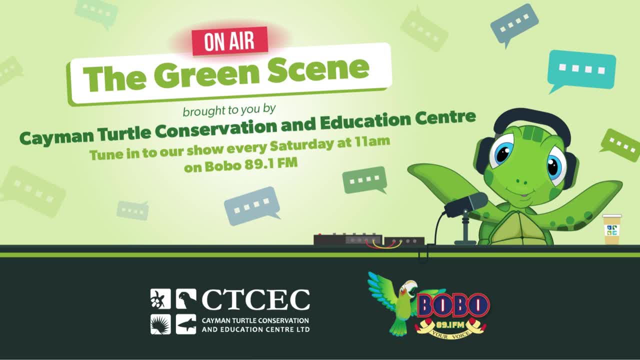 It means you have to do your own research and keep yourself up to date, right, Yeah? and facts and figures can constantly change, So you have to constantly update that information as well. Lots of research, Okay, Okay, guys, that sounds like a lot, but I'm just going to wrap up this section here. 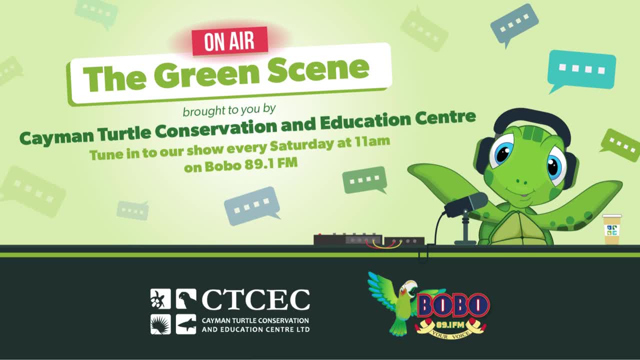 But before we go, I just wanted to ask a couple- just both- a personal question. What is it like? what's the thing you like best about doing education programs? For me personally, it's the look of interest on people's face. 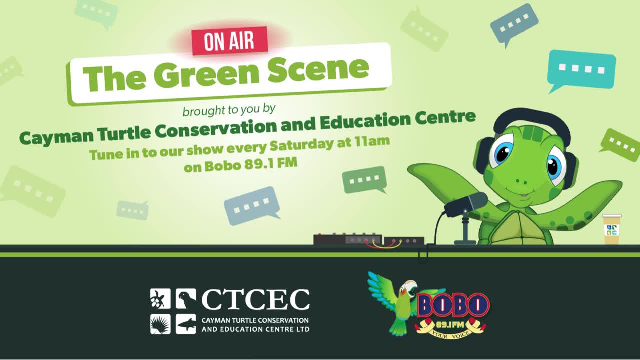 We get some really good visitors every day. Short talk: usually we will alternate: One officer does short talk, one meet, the other does it the next week. So when it's my week, I really look forward to it, because we get some really good visitors each day. 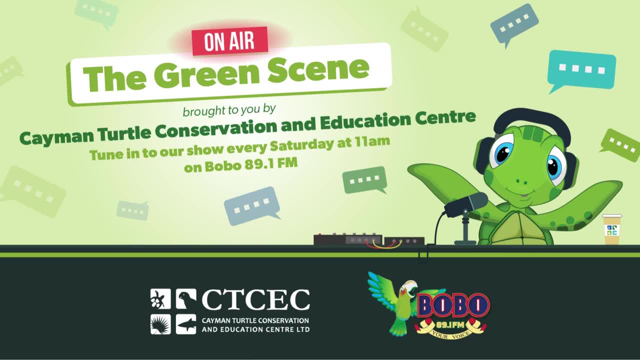 and the enthusiasm on their faces and how their faces light up with questions. it just makes it all worth it. It makes my day before 12 pm. Yeah, and I'll say, the difficult part for me about that question is when you say the word best. 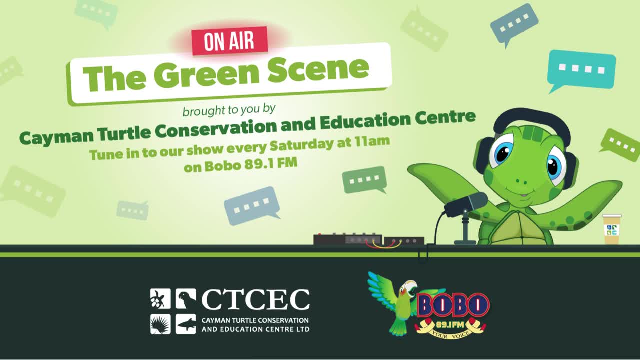 because, as for putting something at the top, I don't know. As I mentioned earlier, my degree and my background are in the animal care field, so I obviously really like when I get to work closely with the animals And educators do, at certain points, get to work very closely with them. 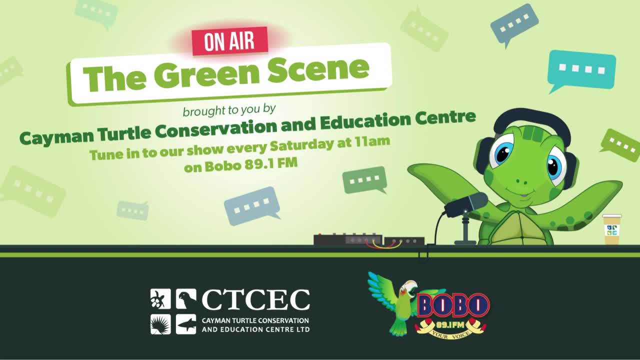 So whether I'm In our aviary talking with one of our parrots like Coco, or whether we're at the turtle releases, that's fun. But also part of the reason I jokingly fell backwards into the education career is that I really genuinely like seeing how kids especially react with learning the information. 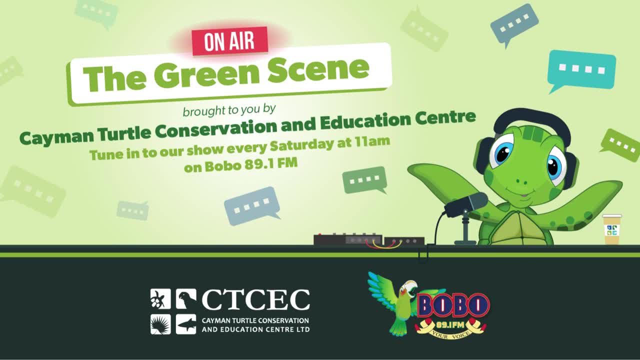 but also just how passionate the younger generations, especially now, are about the environment and the animals, And they're very inquisitive And really love learning things. So that's one of my favorite part: just seeing the genuine joy on their faces. 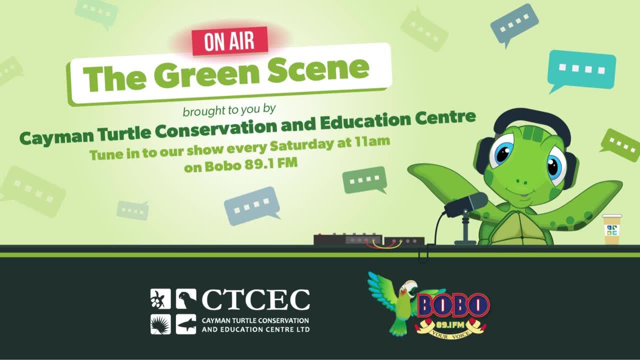 when they learn about these animals and also see them. I will admit, I think Shona definitely has more of affinity for children than I do, whereas I love adults and adult conversation, So it's a pretty good team. It works out quite perfectly. 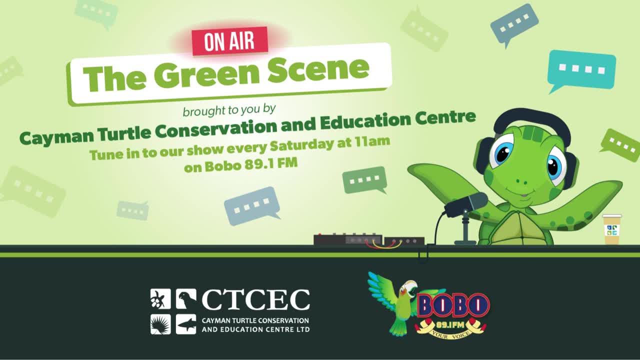 Okay, yeah, balance all around, But the key thing is you have to enjoy what you do, because you're not teachers as such. No, But important, Yeah, Yeah, Yeah, Yeah, Yeah, Yeah. Important information, Information presented with passion is something that's always better retained. 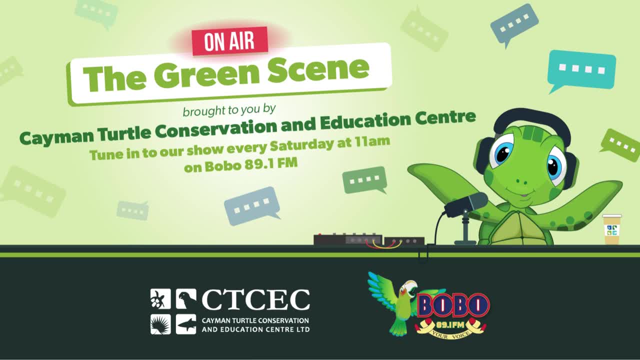 rather than just give a dry lecture. Exactly As anybody who has been to university knows, you might have some brilliant professors, but they're not that good at teaching. Just because they're smart doesn't mean they can impart Well. guys. thanks so much for sharing that information with us. 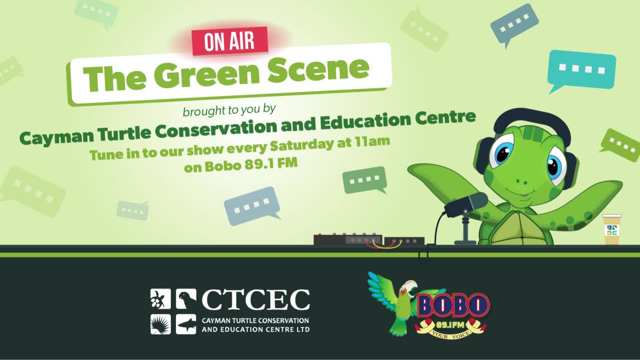 We've been talking with our education programs officers, Wendy Dandy and Shona McGill. on the green scene. We're going to take a commercial break and when we come back we're going to talk a little bit more about how the different departments of the Cayman Turtle Conservation Education. 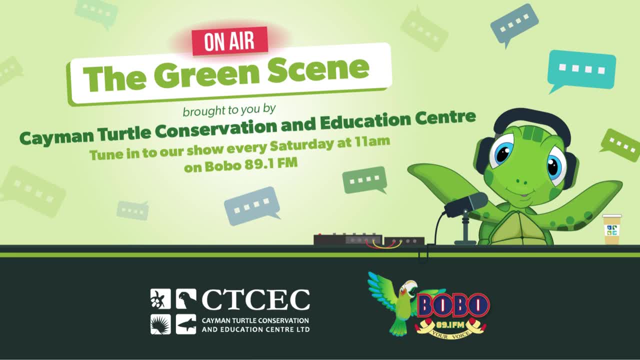 Center work together as a team to contribute to the whole program, the whole conservation mandates of the company. So listen to the green scene here on Bobo 89.1 FM. We'll be right back. Hi, I'm Jennifer And you're listening to the green scene. 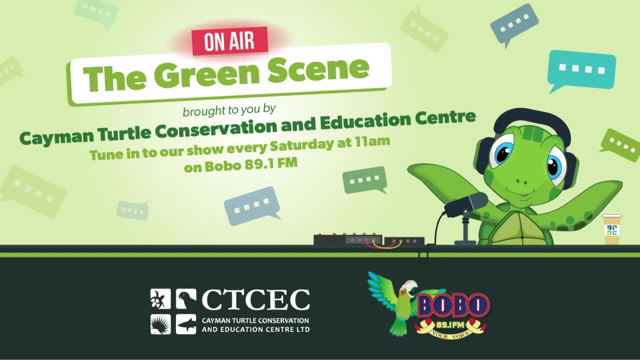 We'll be back in a couple of minutes. Looking for something fun and different to do with the family. Join us at the Cayman Turtle Center for Grill and Chill Saturdays. Every Saturday, from 11 am to 3 pm, Enjoy a poolside barbecue, buckets of beer and daiquiri specials and a live DJ. 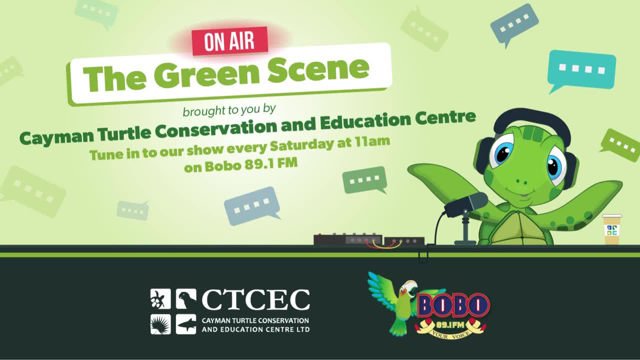 It's Grill and Chill Saturdays at Cayman Turtle Center. Come and celebrate Cayman's culture and our national heroes at Cultural Day at the Cayman Turtle Center. Monday, the 22nd of January, Cayman Turtle Center will be celebrating from 10 am to 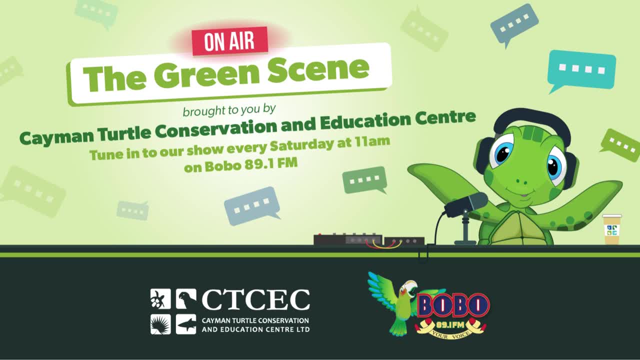 4 pm with incredible deals For you and your family. Come and enjoy food and drink specials all day long. Swim with the turtles and fish in the lagoon, Enjoy the live DJ poolside and have fun with cultural activities throughout the park. 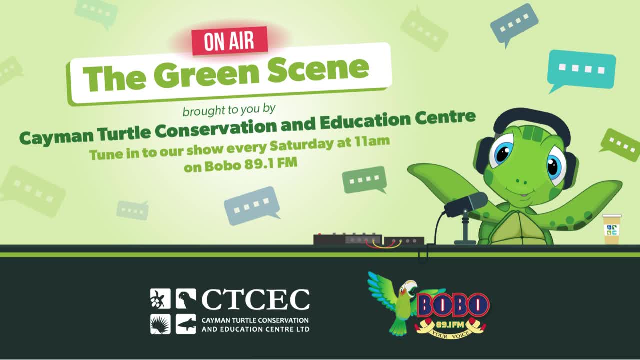 Come and celebrate our heroes and immerse yourself in Cayman's culture at Cultural Day at the Cayman Turtle Center, Monday, January 22nd. Okay, everyone, Welcome back to the green scene on Bobo 89.1 FM. If you have been joining us from the beginning of this conversation, you might have noticed. 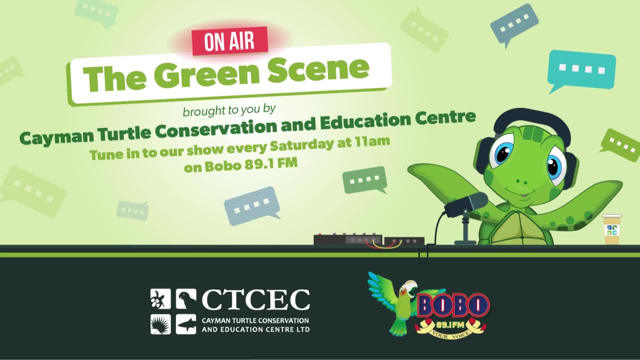 that The host voice sounds slightly different. My name is Shona McGill and I'm one of the education programs officers, and we've sort of switched host seats midway through because next up we're going to talk about our terrestrial section. 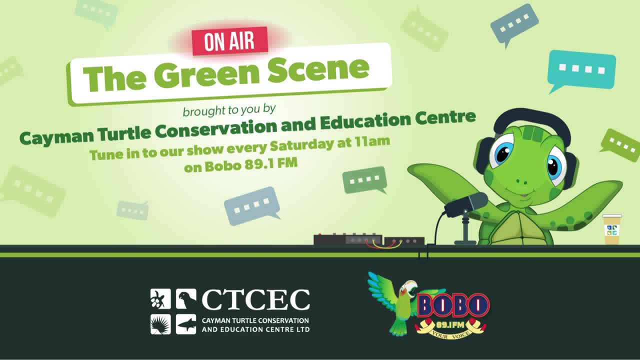 So with me today I have Mr Geddes Hislop, who is the curator of terrestrial exhibits and educational programs at Cayman Turtle Conservation Education Center. So I'm going to first start off by asking you: what's your background And how did you become the curator of Cayman Turtle Center? 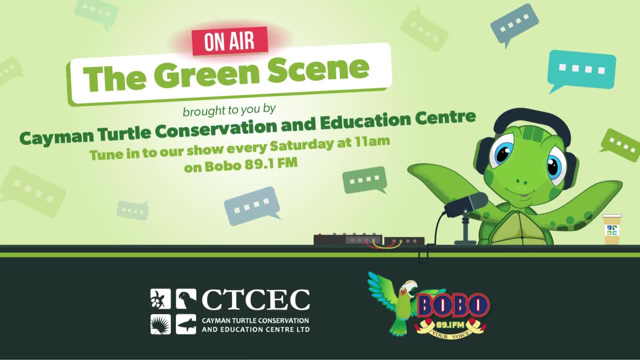 Well, terrestrial department at Turtle Center, although sometimes it feels like that. Yeah well, my background is: I'm originally from Trinidad. I did education. I finished my high schooling in Toronto, Canada, and I went on to get a degree in wildlife. 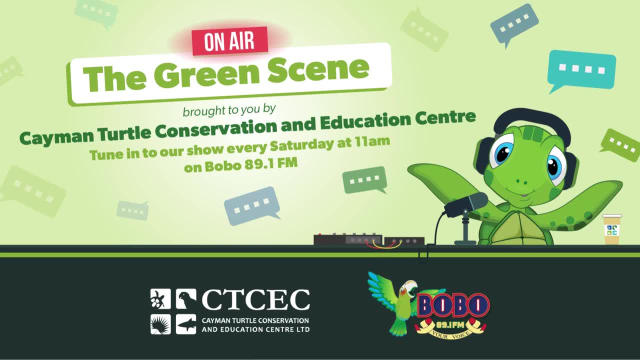 biology with a minor. I was a senior in environmental education at the University of Guelph, which is well known to a lot of Canadians, And from there I went back to Trinidad and I worked in wildlife conservation and research with the Trinidad Wildlife Department and then eventually moved to the Cayman Islands. 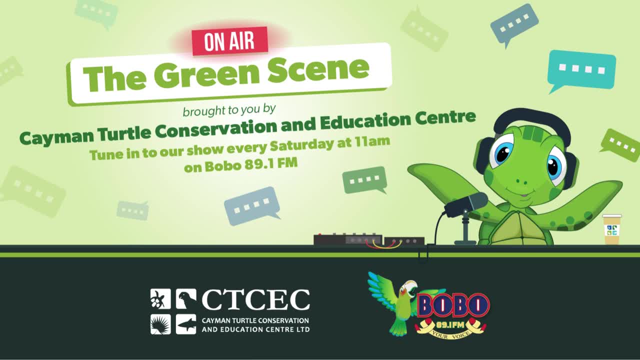 Worked with the National Trust for a while as an education programs officer, and that was the time that we opened in the early days. And then I was recruited by the Turtle Center back in 2006,, 2005,, when they were just opening. 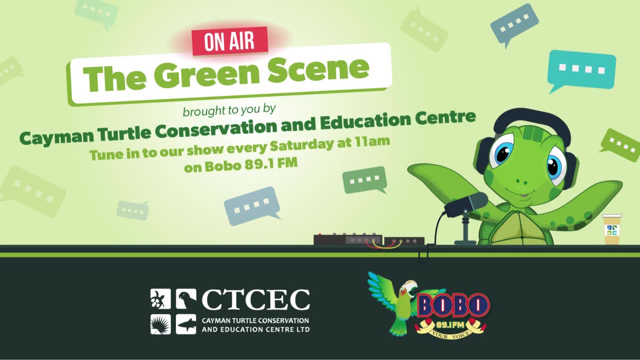 up the new Boston Beach. they called it at the time And, yeah, the education programs and the terrestrial department grew from there. So I'm sure most people know about Cayman Turtle Center. We definitely have turtles, But it's a lot more animals than the turtles. 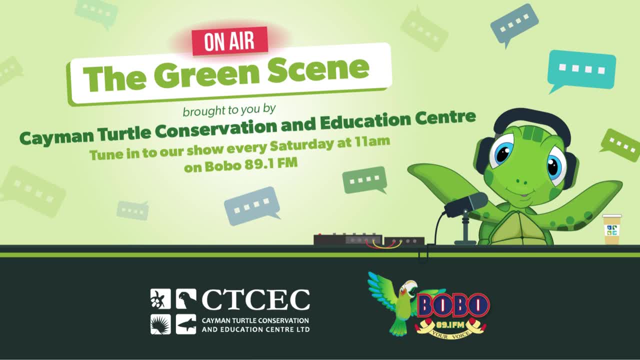 It's a lot more animals than that which is also where you come in. So you jokingly say you work with anything with legs at the center. Yeah, Anything with feet. Yeah, Because we have from butterflies to a crocodile, And but the main focus most people know at Cayman Turtle Center is the aviary, the Caribbean. 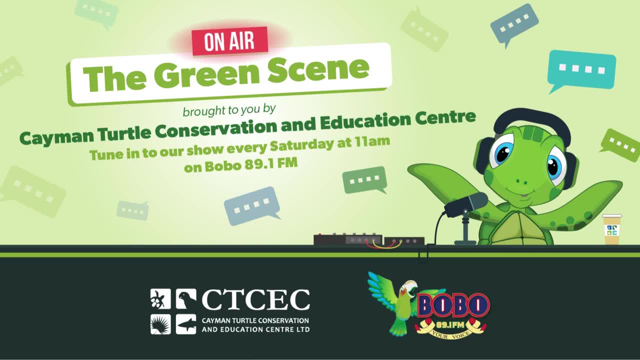 aviary. That's the main focus. And at the Turtle Center there's conservation going on all the time and we actually do conservation. We have dedicated conservation programs for three species at the Turtle Center: the green sea turtle, of course, as Dr Navi had discussed earlier. 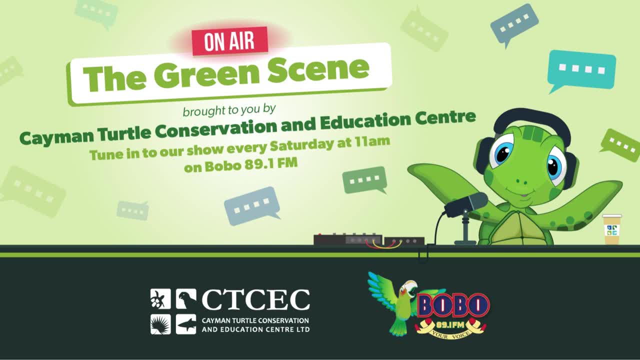 And we also work with another iconic species, another national animal, which is the Cayman Island parrots. Parrots- And I just say parrots, plural, because there's two national birds which are the two Cayman Island parrots: the Grand Cayman Parrot and the Cayman Brack Parrot. 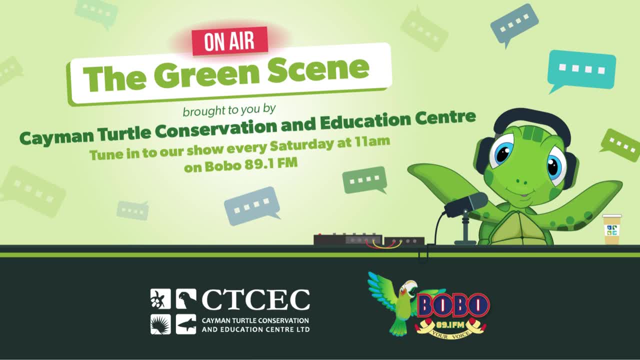 So the Caribbean aviary, The Caribbean aviary at the Turtle Center, is the only place in the world where you can see both subspecies side by side. So one of the things that we do is we teach people how to tell the difference. First, we tell them there's two parrots. 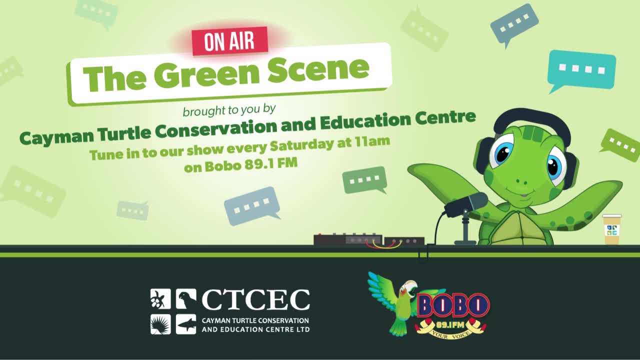 So the thing that we'd like to do is say, yeah, well, we have all these, this bird and that bird, that bird, and we have the two national birds, And then pause And everybody says: wait what? We have two. 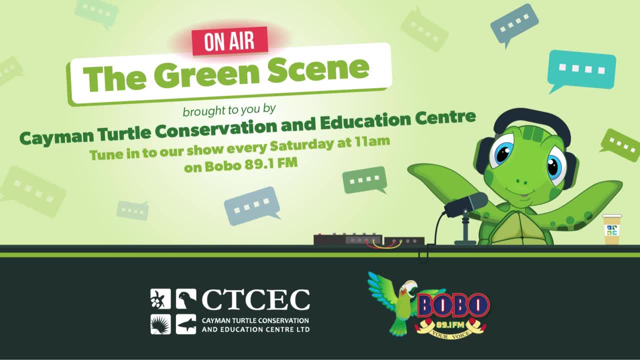 So, yeah, So we have two national birds, the Cayman Island parrots, Two national, the Grand Cayman Parrot and the Cayman Brack Parrot, And they're both because the official, the official national bird on the government website. 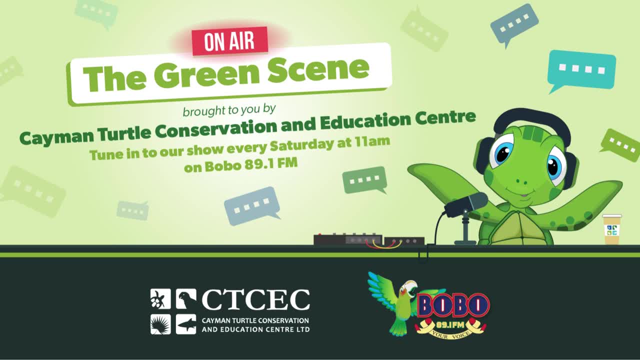 is the Cayman Island Parrot, And there are two Cayman Island parrots, So they're both equally national birds. And then, apart from that, we also work with the white-crowned pigeon, which most locals might know as a bald-pate. 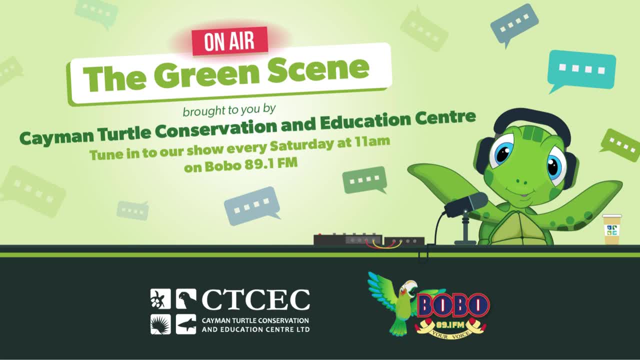 We started that after Hurricane Ivan because they've been, because their numbers plummeted after the hurricane, of course, And they're in big trouble. So we, and we got a lot of rescue birds at the aviary, We do some rehab, I should mention. 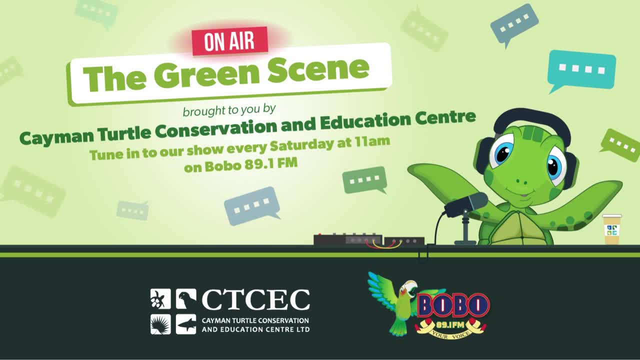 We don't. we try not to take wild animals in because of the general park policy about for biosecurity, where we don't want to bring disease into the park, But in some cases we do. we do have some animals that have been cleared by the vets that we 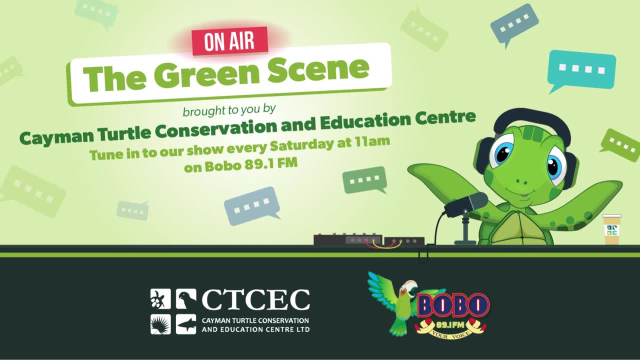 rehab And when you're rescuing injured, injured, wild white-crowned pigeons. We had white-crowned pigeons after the hurricane. They stayed in the aviary and as they got better they started breeding And we figured: well, this is a good way to help help the population make a comeback. 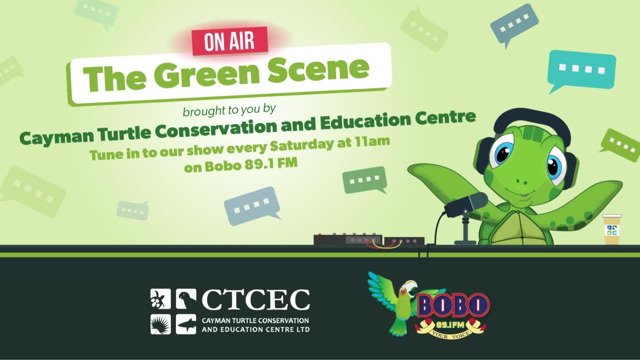 It seems over the years that the population of white-crowned pigeons has made a good comeback. But yeah, besides the aviary, there's also most. there's also a butterfly house, and it's not a butterfly farm. We're not breeding butterflies. 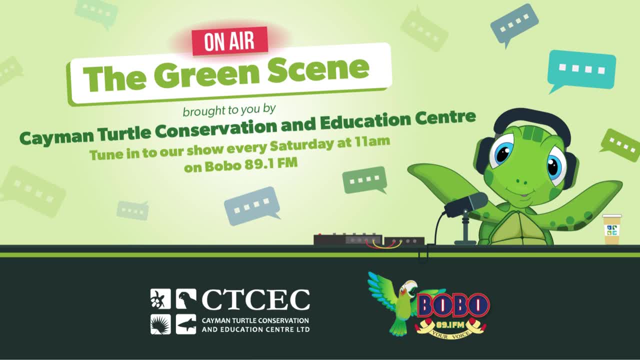 It's. it's basically an enclosed butterfly. It's an enclosed butterfly garden, So people get in there and they can see local butterflies. One of the things that interesting is that people walk in there and they say I don't see any butterflies because they're not moving all the time. 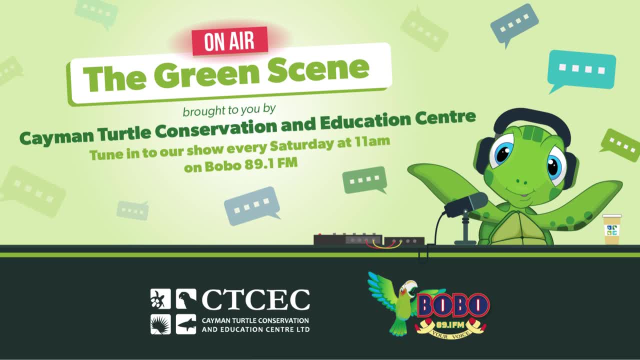 And once they stop moving, they just disappear. It's the same thing as, say, in the aviary. sometimes people walk through the aviary. I don't see any birds. They're in the trees. They're in the trees. First you got to look up and then you got to slow down. 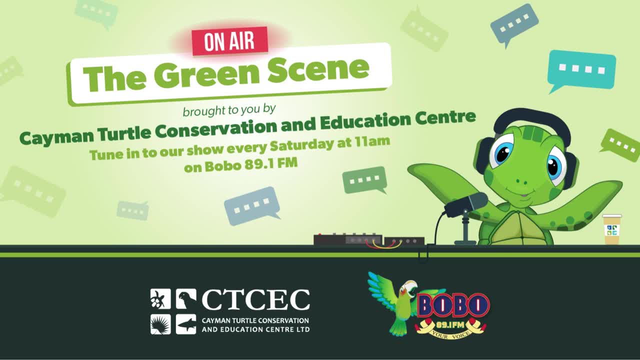 Yeah, You know. so it's you know. I tell people that you know it's like when you look in these wildlife shows you get a 30 second clip that probably took them about three months to get. Yeah, They're not active 24 seven. 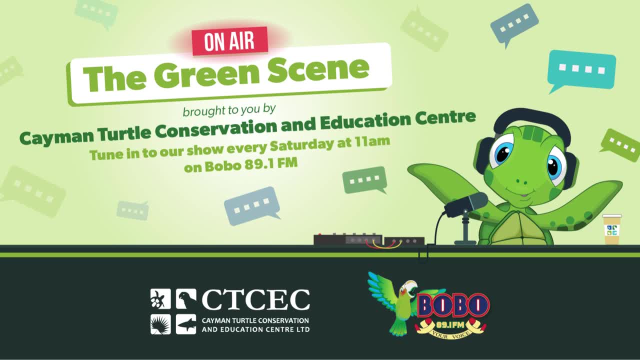 Yeah, And then, of course, on the on the islands and the big lagoon, the snorkeling lagoon, we have our peafowl on the islands. They're there mainly for entertainment and attraction. There's a nature trail in the back there. 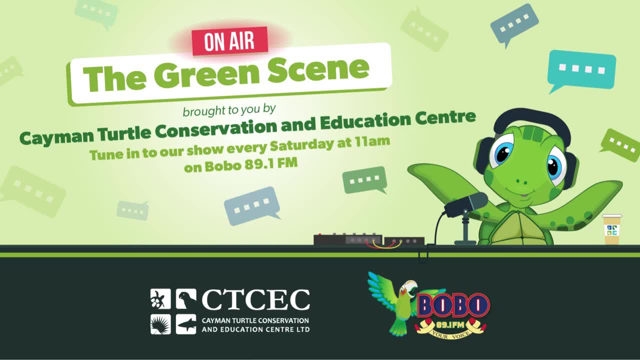 Because we Besides- Yeah, Terrestrial- also involves plants. So we do have a small nature trail in the back there where people can enjoy a nice, quite a nice short walk through the woods, but it ends up at the blue hole cave, which 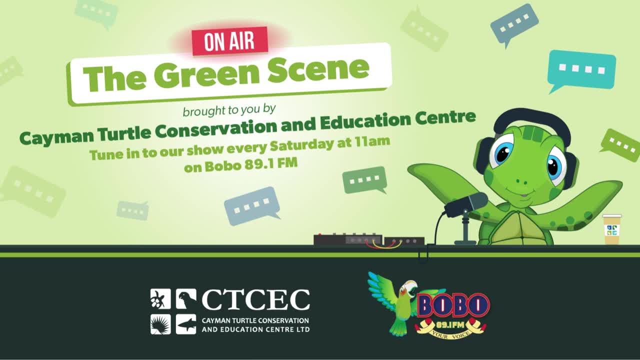 most people don't know about, but it's like there's an actual cave on site, Not that you can walk into like in the BRAC, but you can look at it from a, from a distance. And in that cave there's a certain, there's a certain type of blind cave shrimp. 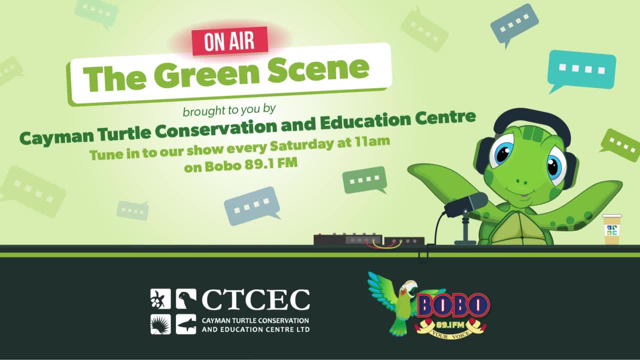 It's not microscopic. We can see them in the naked eye. but there's a little white cave shrimp. that's unique only to that cave. You can't find anywhere else, And we do have researchers that come from from the US every year to study these things. 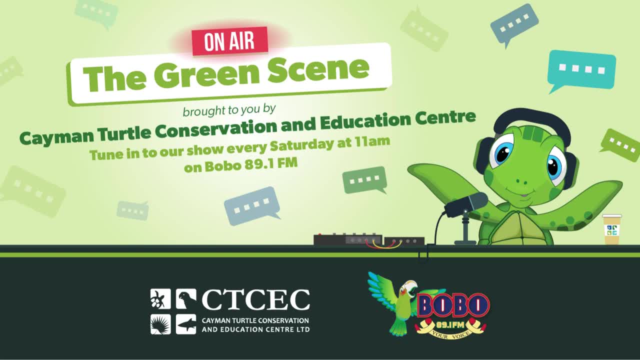 And then, of course, we have our crocodile. Yeah, Yeah, Smiley the crocodile. Most school kids knows, know about Smiley and we feed her once a week. So yeah, Right now In the wintertime, we feed her once a week, usually on a Wednesday. 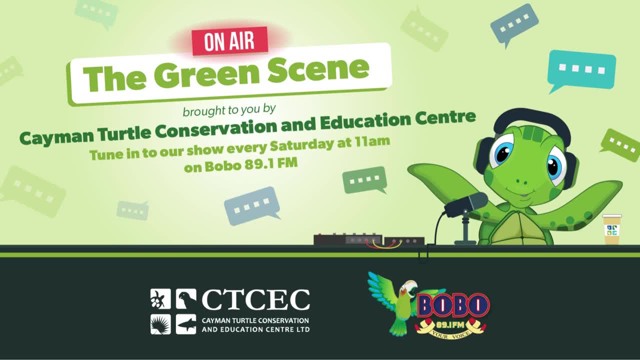 In the summertime we feed her twice a week. odd times might feed her three times a week. That's pretty much the education programs, sorry, the threshold programs. So if anybody has been listening very, very closely to Geddes, not only has he mentioned 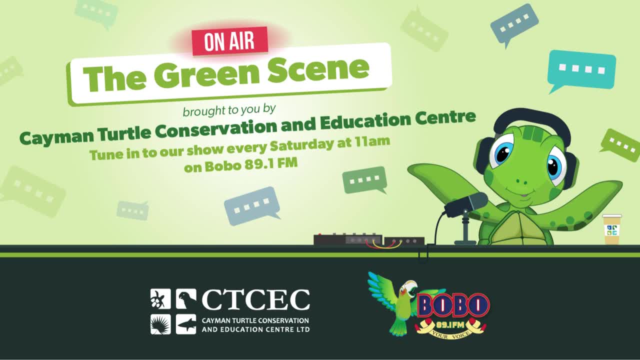 multiple species, but he's also mentioned multiple habitats at the center too that fall within his realm, And it's a very common misconception that when you work with animals, you just spend most of your time cuddling them. We do not just cuddle animals 24 seven. 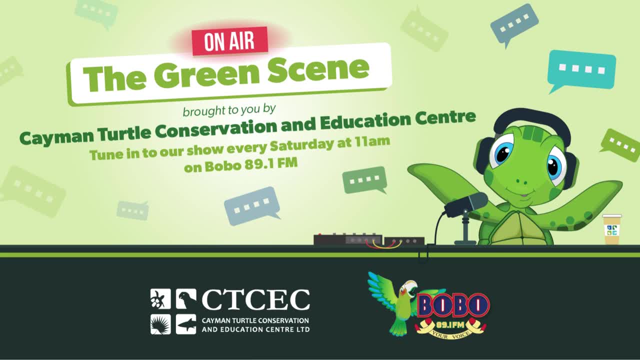 Definitely not the crocodile. There is a lot that goes- definitely not the crocodile. Yeah, There is a lot that goes on behind the scenes. So how would you typically describe a regular working day for you and your department? Yeah Well, myself and the other keepers. 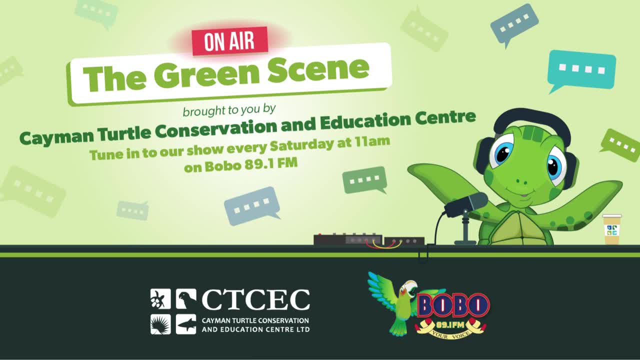 Yeah. So let's say we spend about maybe half of our day is feeding, cleaning and observation- Those three things These animals are taking. they're not pets. Make that quite clear, Because most people when they come in to the aviary, especially when they see the parrots, 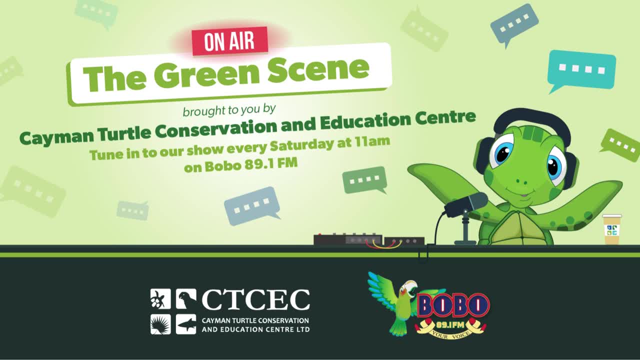 first thing they want to do is: does it talk? Can I pet it? No, they're not pets. We don't treat them as pets. We actually want them semi-wild Because, because of the breeding and release program, we want them to be able to to be. 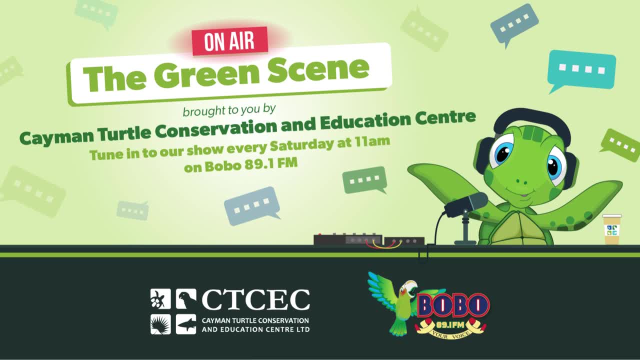 able to quickly adapt to living in the wild. So we don't treat them as pets. So I tell people that they're tolerant, they're not tame, They'll let you get close. They don't want you to touch them. So because we have these wild animals in a controlled environment, they cannot move around. 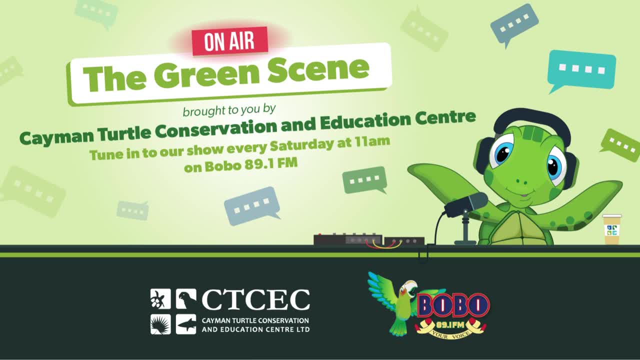 as they would in the wild, and they cannot access certain things, So we have to make sure that they're that they have All their basic needs provided, So feeding and cleaning is is an important part of it, because animals don't like dirty. 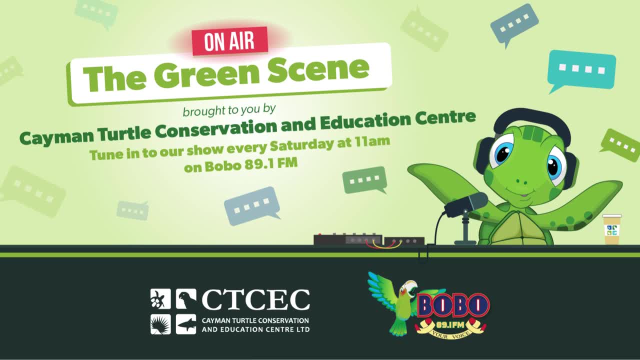 stuff anymore than we do, And if there's something dirty, usually they just move. But since they can move, we've got to make sure that their, their, their environment is clean, And that's good for health too- health and welfare. 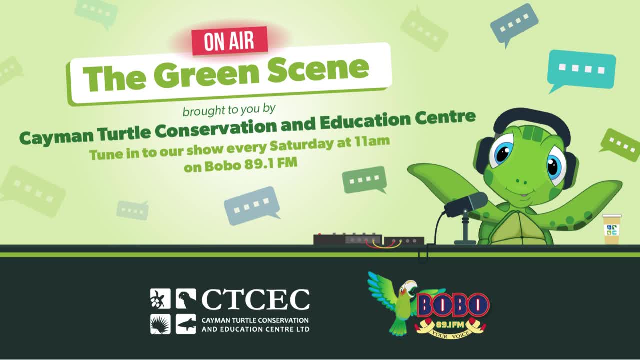 Feeding them is more than just putting food in a bowl. We have to. we actually give them portions. We try to give our animals as much of the natural food as we can Because we believe there is a commercial, special diet- zoo diet- that we get that the 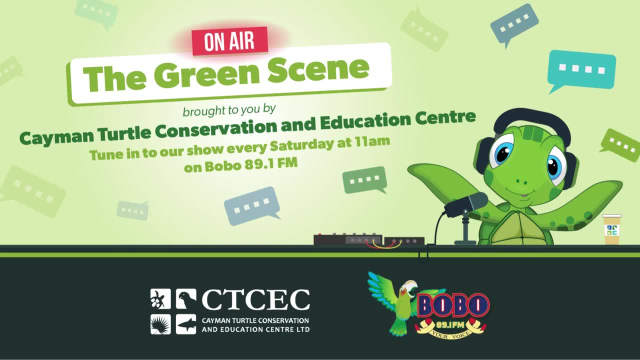 that provides a hundred percent nutrition. But we believe that there are certain. there are certain nutritional qualities in the, in the food that they eat in the wild that is not accounted for. you know, just like you know when your mom tells you eat your vegetables, vegetables, she's not saying that. 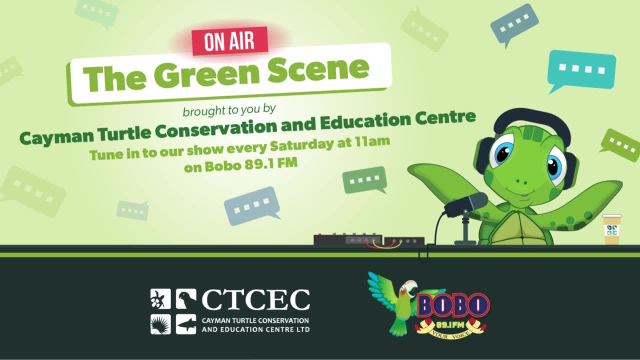 because, just for so, because there are certain nutrients and vegetables and different things that are that are good for you, that you may or may not get just eating a pizza. So so we try to give the animals as much natural food as we can. 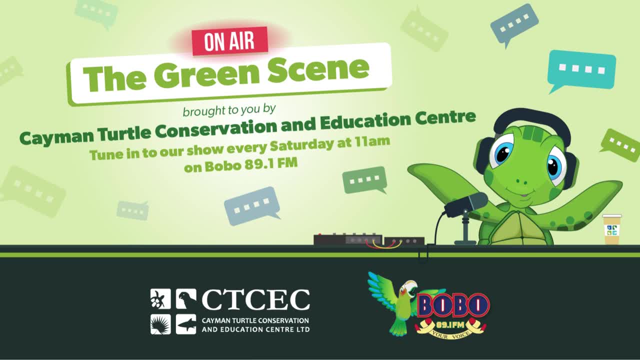 So part of this is they will normally go foraging for food. We forage for their food. So you see our, our guys, walk around picking up almonds, you know, picking fruits from different places, even flowers, you know. uh, the cleaning is an important aspect, as 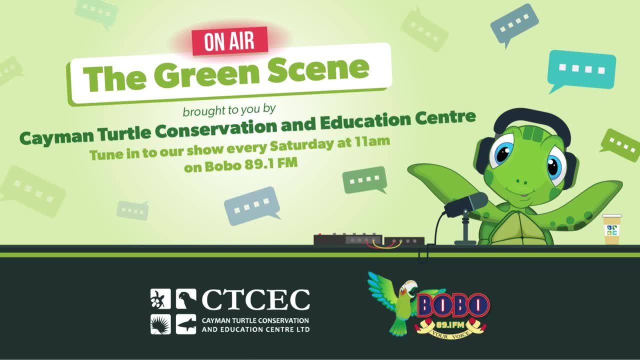 I said because you want to avoid. you want to avoid, well, not just mess but also in, you know, possibly the animal, in attracting unwanted visitors, like, like bugs, just because there's a lot of food that attracts ants, or something like that. 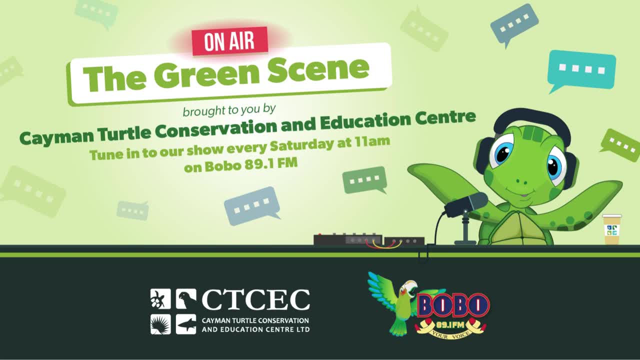 And then observation. again, these are wild animals. They don't animals. in the wild they tend to hide any kind of illness or injury because otherwise they're targeted by a predator as an easy prey. So these animals will. if they're injured or sick, they will hide it as best as they. 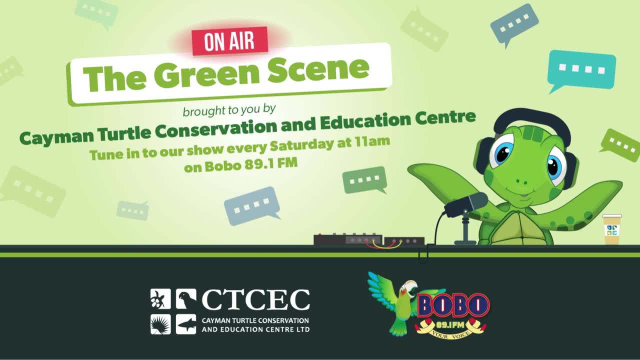 can. So by the time they actually show any kind of any kind of ill illness, it's usually at a really advanced stage. So, again, the keepers are trained and and experienced in looking at animals and learning what is, what is normal behavior? uh, just like our vets mentioned, and if anything is, 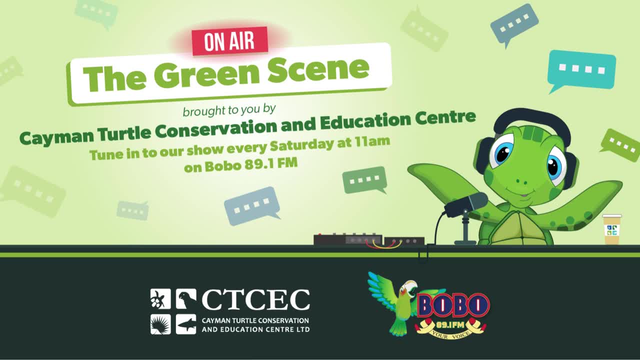 abnormal, we flag it right away and you know we look at it a little closer or, if anything, we contact the vet, Dr Navi, to get a, to get a better assessment. So all this is part of the welfare. 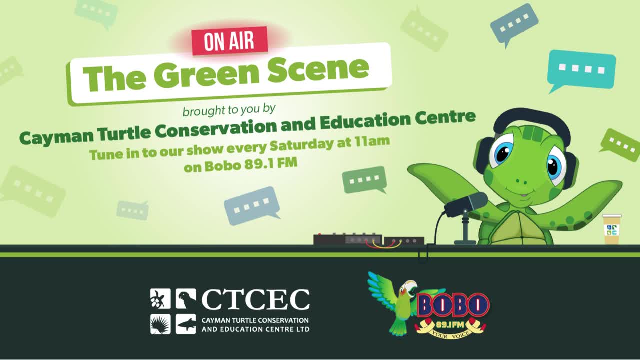 Yeah, That's a top thing. What you most visitors see is it, is it the benefit of that? They see animals that are happy, healthy, moving around. you know, bright and active or, as like we, we like to say, bright, alert, reactive. there's a lot of work that goes. 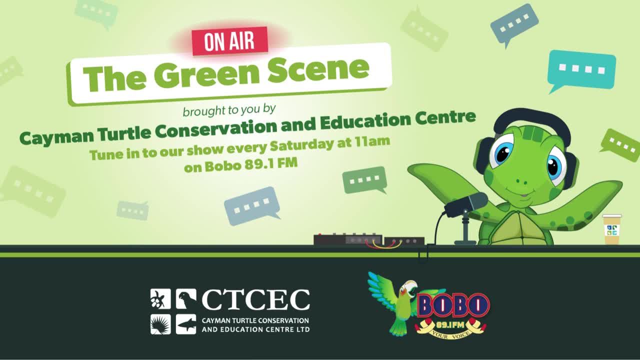 into it. Yeah, You, you said you guys have to be really good at noticing the behavior of animals, because they don't display outward symptoms. Yeah, Yeah, Yeah, Yeah, Yeah, They don't display outward symptoms. but it's not just that. 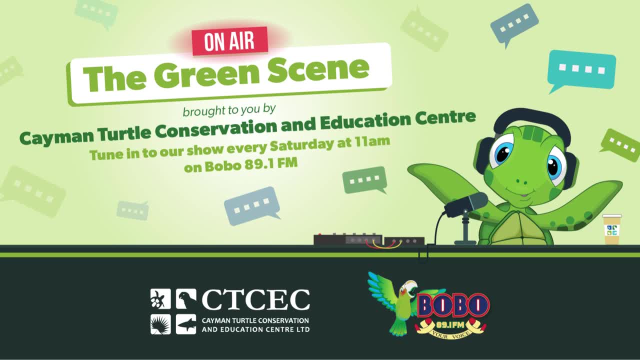 You also have to study individuals too, because just like us humans have our own specific, unique traits, so do all individual animals as well. Oh, yeah, Yeah, Because after we we don't name all the animals, but some of them we, some of them we know. 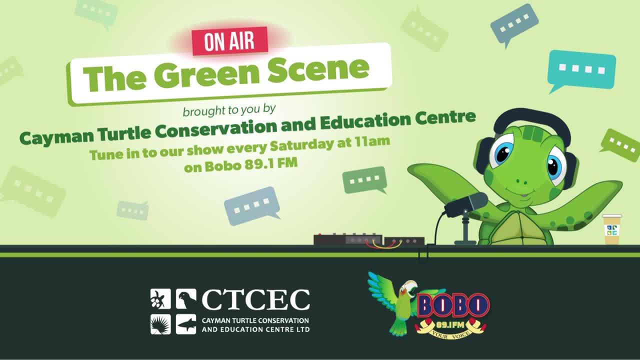 individually, as you said. And uh, and yeah, those animals are, are iconic to us. Uh, we know. for example, all the parrots are named right And Smiley. this crocodile, of course, has a name. 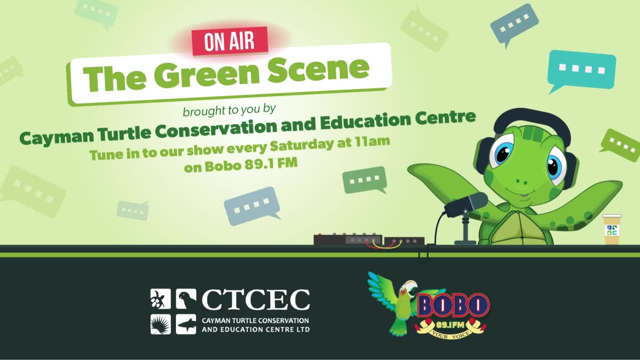 Not the name I would have chosen, but Smiley sounds friendly. Well, she's not that friendly. So even some of the pigeons and other birds have names. So yeah, and that's another thing When you're working with animals close to that in captive situations. 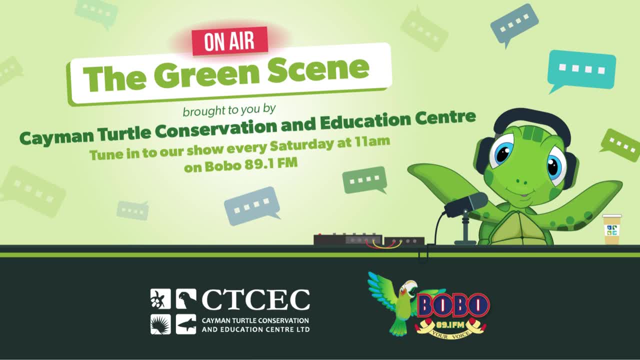 it gives you an insight into what they're like in the wild Because, for example, with the Department of Environment doing their field research, it helps if they see certain behaviors and they can discuss it with us And we can tell them. well, yeah, this is something we've seen our animals doing as well. 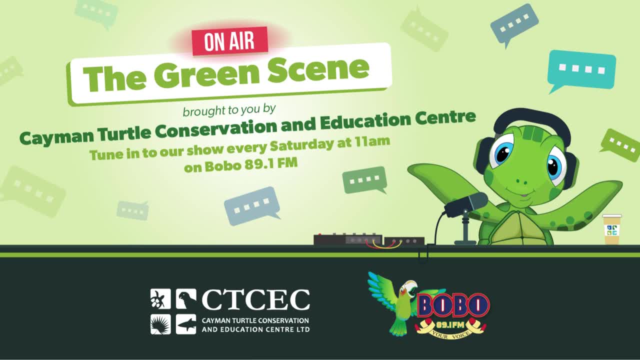 So they have a better idea of how they can manage certain things If they see, for example, feeding on certain things at certain times of year. So we're working with wild animals in a captive environment And for us, in that scenario, there's a lot of stuff that goes on behind the scenes. 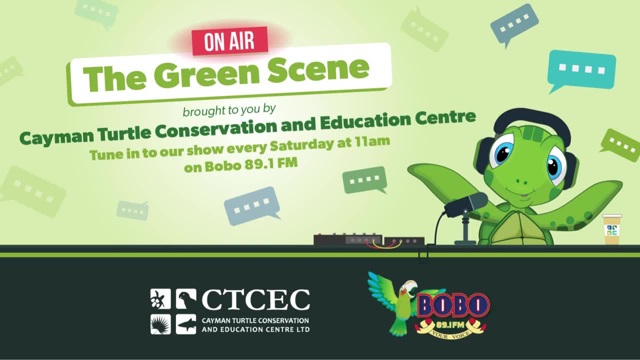 But especially something called enrichment, which is actually very beneficial to the animals in our care. So can you just please explain enrichment and why we also do enrichment for our animals? Enrichment is basically a way to help the animal express natural behavior. Very simply put, it's a way of entertaining the animals. 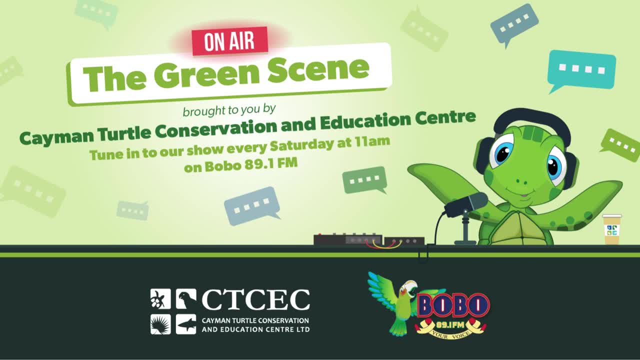 If you're sitting down in a room, for example, and all you have is your four walls, you get brought pretty, pretty quick, pretty quick. They give you a book. Now you have something to do. They give you a, they give you a video game. 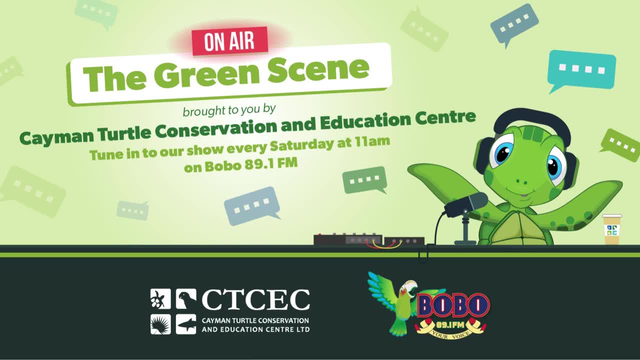 You have even more to do. So in the case of the animals, we try to provide them with enrichment. Enrichment can be something as simple as giving it something, something nice to eat. It could be as complex as changing the environments. 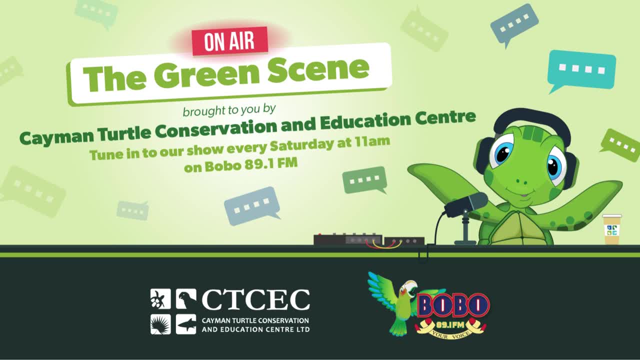 like hanging up branches and so on, Like we do for some of our parrots, changing around perches and moving them to a different location And the aviary. some of our animals interact with the guests with hand feeding. Uh, Smiley the crocodile, her enrichment every day. 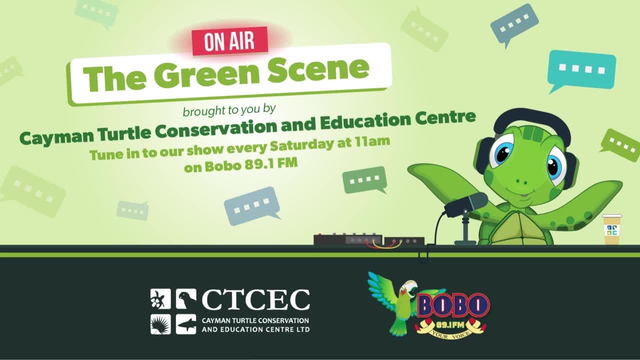 Well, sometimes we spray it out of the holes, but her main enrichment is feeding. That's the time when she gets to move and pursue the prey, which is food on the end of a stick, basically. And so, yeah, enrichment is very important for the animals' mental health. 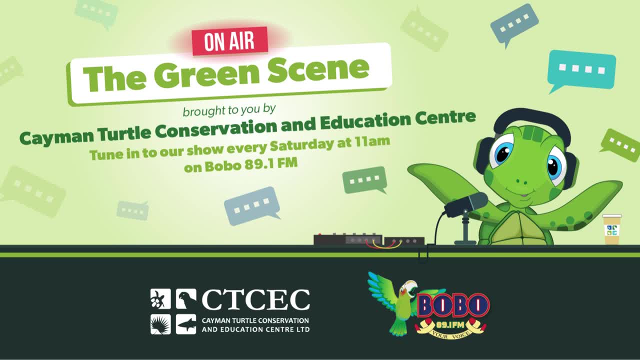 Because anything, if you're bored and you're depressed, you're much more vulnerable to getting sick And so, yeah, so enrichment is a very important part of what we do: Feeding, cleaning, yes, but making sure the animals are happy and healthy. 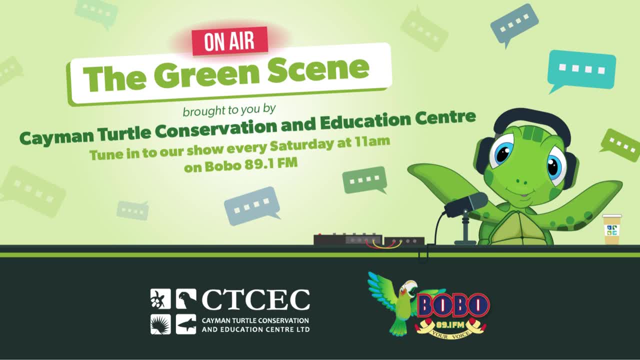 There's another. there's another aspect of it as well, which is enrichment. Well, thank you so much for joining us, Geddes. I do think we have to wrap up. We've talked about a lot of things today and hopefully we've managed to give you. 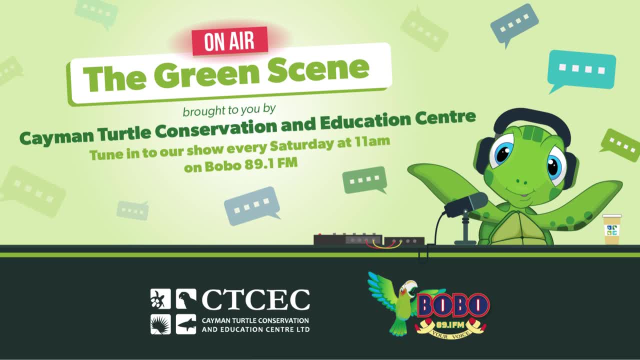 listeners an in-depth look at the animal programs that we have at Cayman Turtle Center. So throughout the week, if you want to see or meet anyone- you may have heard talking today and perhaps ask them more- we have various things going on around the park. 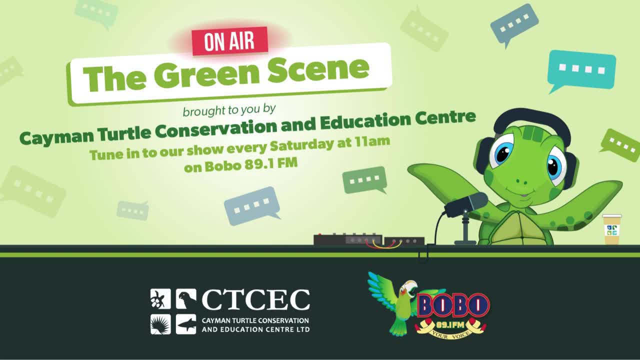 Obviously we have our animal feedings and animal talks throughout the week. So we have shark talk Monday to Friday down by the predator reef viewing glass. that gives people a little more education and awareness on sharks and maybe how they're not the ravenous man-eating machines that media likes to play them as. 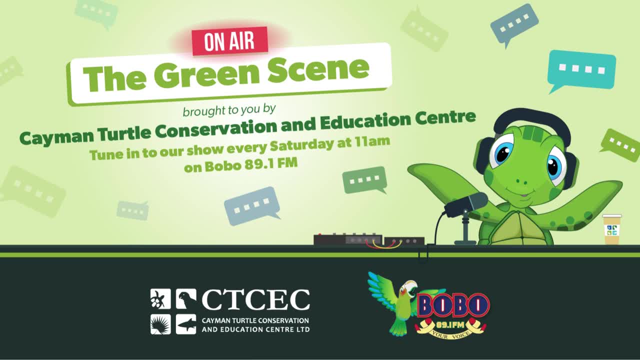 And that's at 1030 down by the viewing glass, Monday to Friday. That's immediately followed by shark feeding, which you can see our two nurse sharks, Freddy and Buka, get fed by our marine department at the center. We do have our smiley feeding throughout the week. 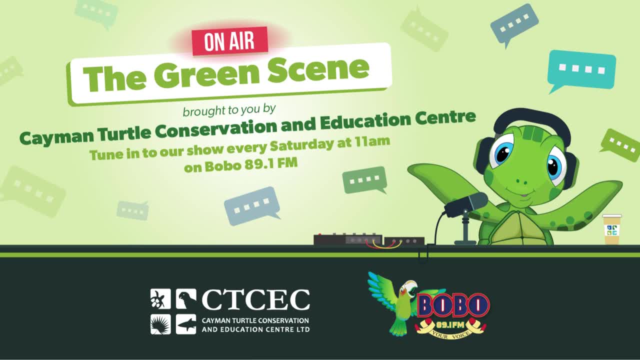 Right now, that is once a week on Wednesdays at 1145.. And then we do also have our Caribbean aviary, which you can visit anywhere between 10 to 3 pm and hand feed some of the birds there. now, as for other things, other unique things that might be coming up at our center, 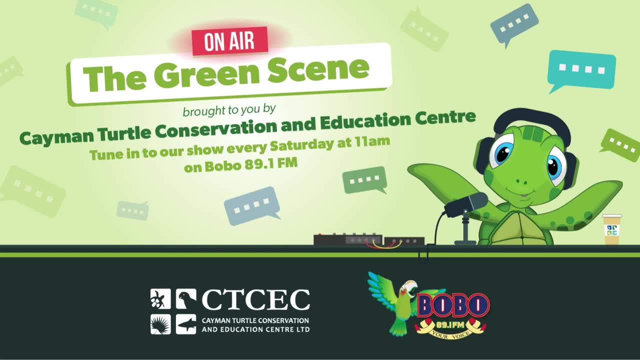 we do have a cultural day coming up, and that'll be on monday, january 22nd, from 10 am to 4 pm, and this will be a really cool event which showcases the talents of local artisans, crafters and also cultural ambassadors. there'll be a live dj beside our pool. there'll also be